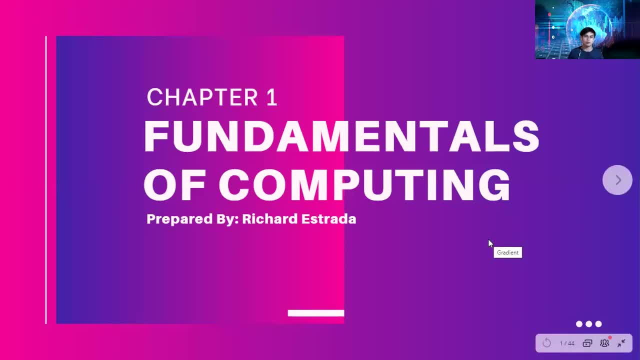 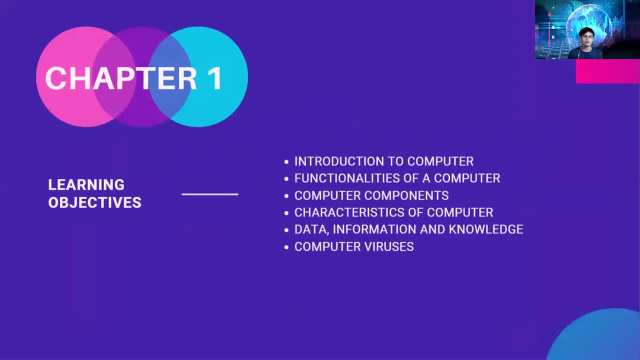 Hello everyone and welcome to our chapter one: fundamentals of computing. Okay, so for this video we will be learning the following. Our learning objectives would be the introduction to computer, its functionalities, the computer components, the characteristics of computer. Of course, we will differentiate: what is the data, information and knowledge, and also the computer viruses. I 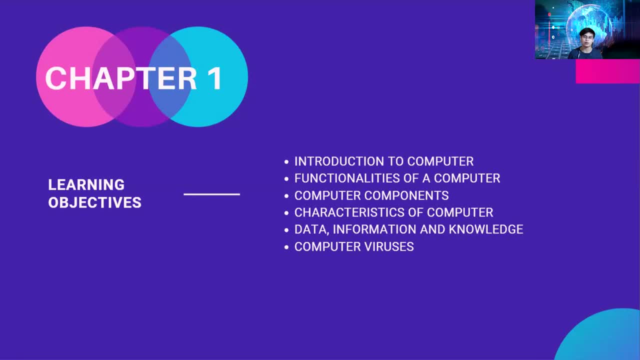 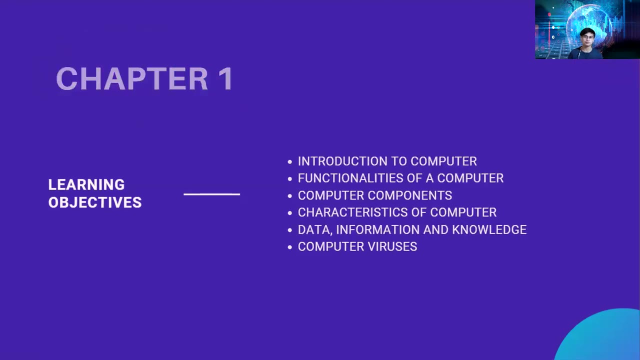 believe you guys have already an idea what a computer is all about. This is just for a recap and also some of I'll be giving you some of the information that you must know about the computers. Okay, let's start with the computer, Of course. computer. 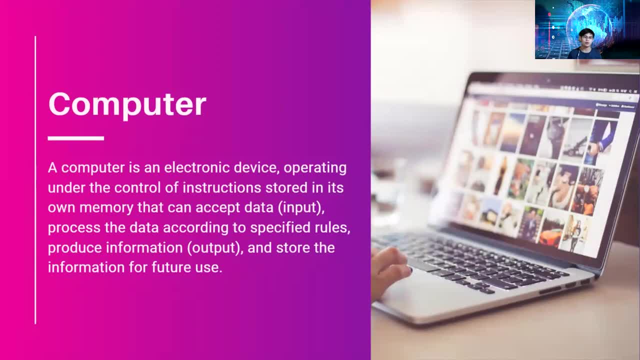 Let's start with computer, of course, Computer computer, Computer computer is an electronic device operating under the control of instructions stored in its own memory that can accept data or the input, the, the process. it processes the data according to specified rules, produce information and store the. 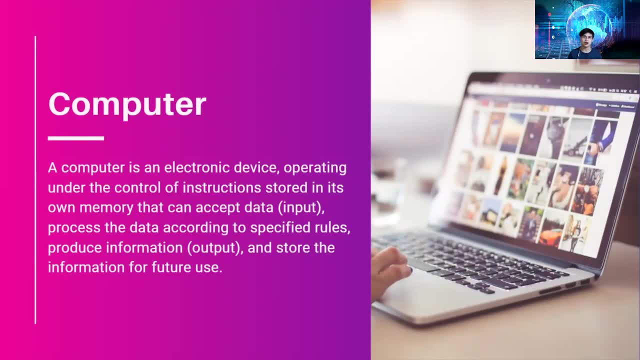 information for the future use. so I believe you have already used computer also. McKee tribute a school, say no, my lay or anywhere. okay, so again it. it is an electronic device that, operating under the control of instructions, stored in its own memory. sorry, yes, 다시, okay. so what is the? 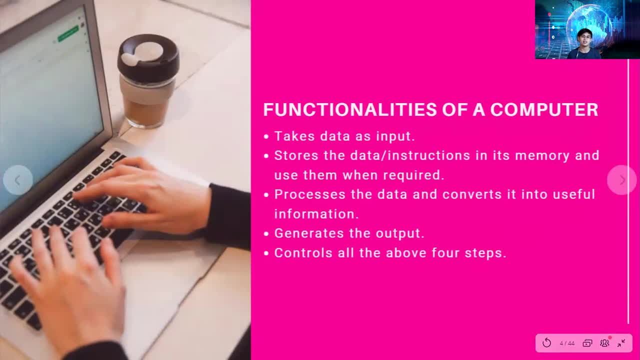 functionalities of a computer. it takes data as input- okay. after taking the data, it stores the data instructions in its memory and use them when required- okay. processes the data and converts it into a useful information and it generates an output and it controls all, all the above four steps. okay again, if we're gonna take the. 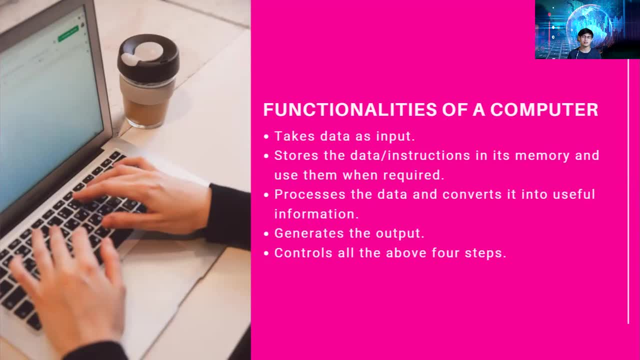 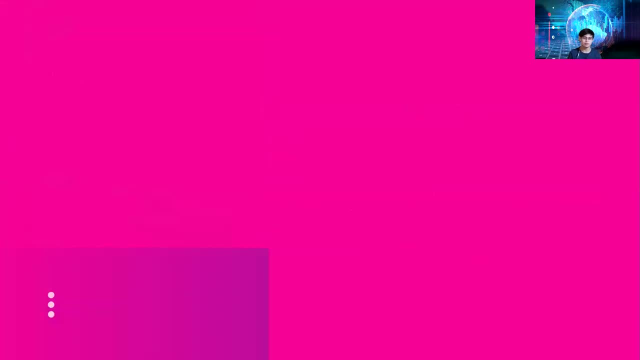 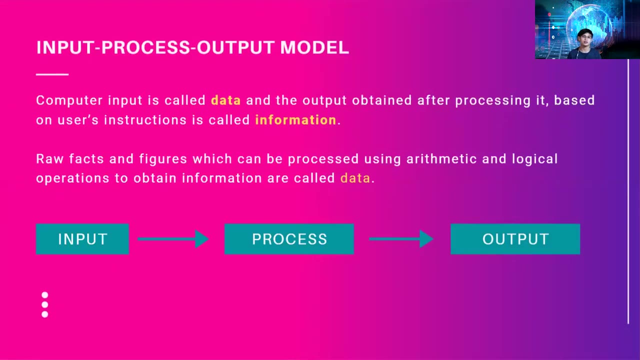 data and we're gonna store the data and we're gonna process the data and generates the output. so, as you see, a step. okay. so that is the functionality of a computer, okay. next, so the computer has this very easy process model. no, it has input process and output. so the user will gonna input, the computer input the. 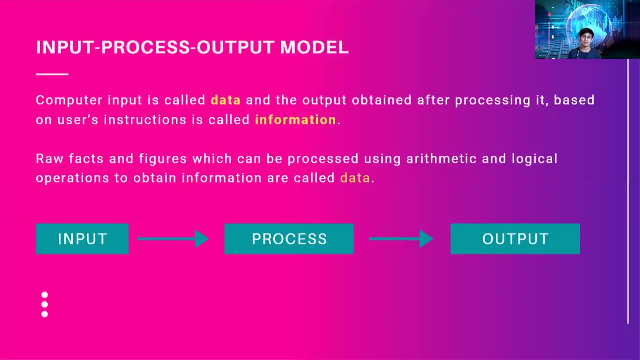 computer will going to process it, okay, and then it provides an output to the user. so the computer input is called the data. okay, if you are using computer, if you the input to it, that's a data, and then the output obtained after processing it based on the user instruction is called information. okay, so let us say for: 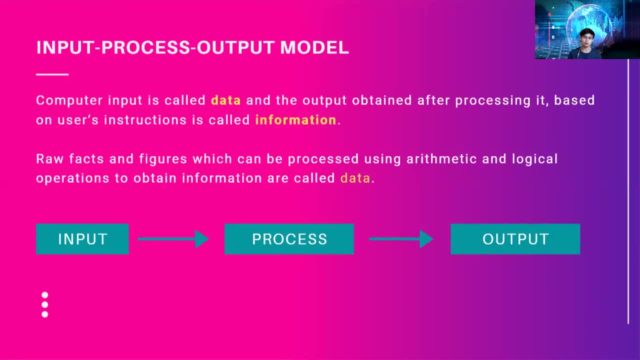 example, I click on the Google Chrome. you know you provided an input to your computer and then the Chrome is open and then you search into it and then the if we're gonna give you the information, something like that. it's just a basic description about the input process, output model. okay, real facts and figures. 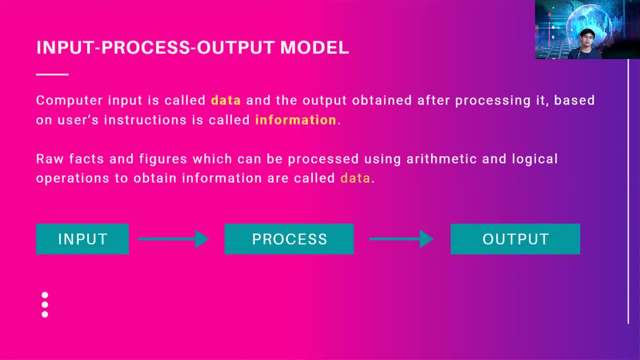 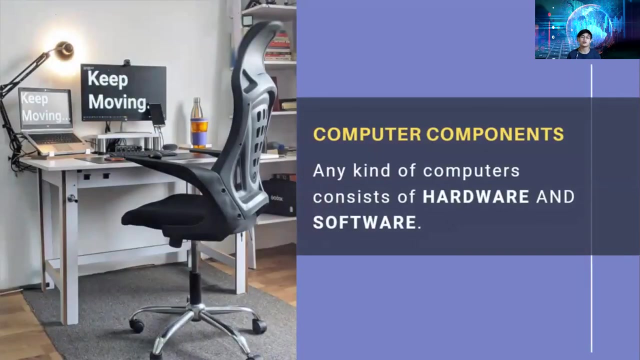 can be processed, or using arithmetic and logical operations to obtain information, or called also data. so you can again, it's a very easy. no, it's just a user will get input something and the process then it's- we're gonna give you an output- is the simple motor of a computer. Next, what are the different components of a? 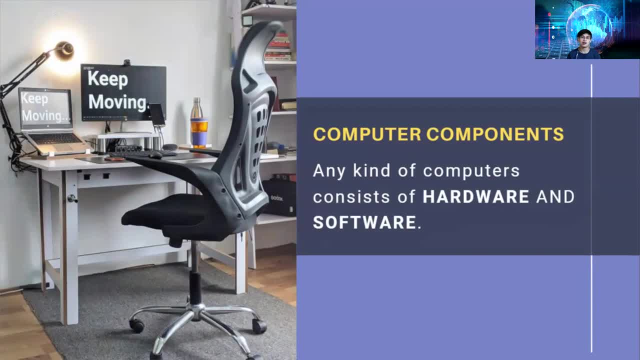 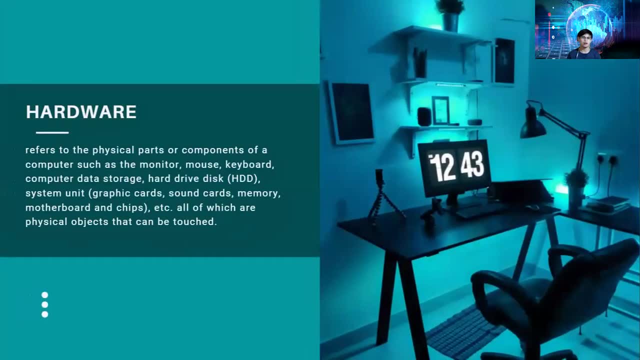 computer. A computer has, of course, a hardware and a software. Okay, so what is a hardware? A hardware? it refers to the physical parts or components of a computer, such as the monitor, the mouse, the keyboard, the computer data storage. 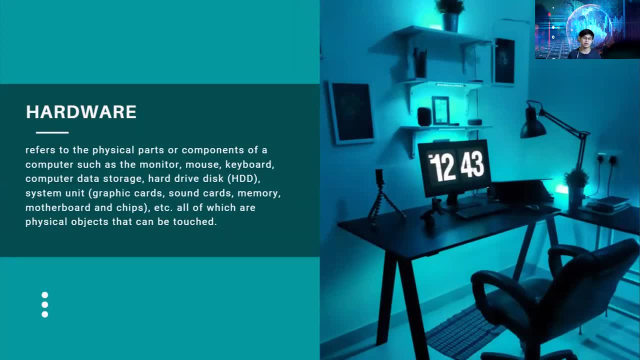 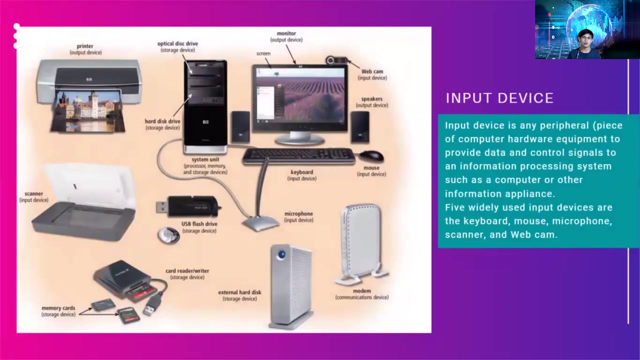 the hard drive, disk or HDD, the system unit, the graphic card, sound cards, memory motherboard, etc. All of which are physical objects that can be touched. Okay, so that is hardware. I believe this is very understandable because you've been using this all the time. Okay, so a hardware has input device. 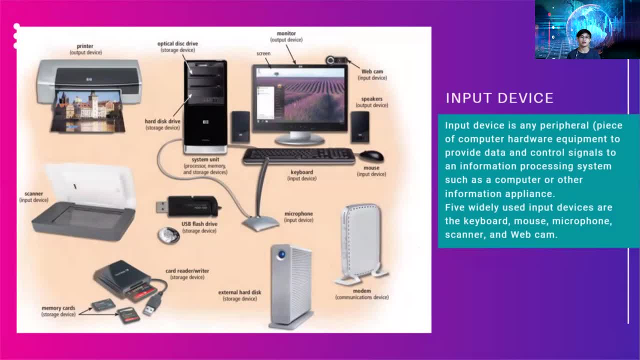 device and output device. For the input device, what is an input device? It is any peripheral. Okay, it is a piece of computer hardware equipment to provide data and control signals to an information processing system such as a computer or other information appliance. 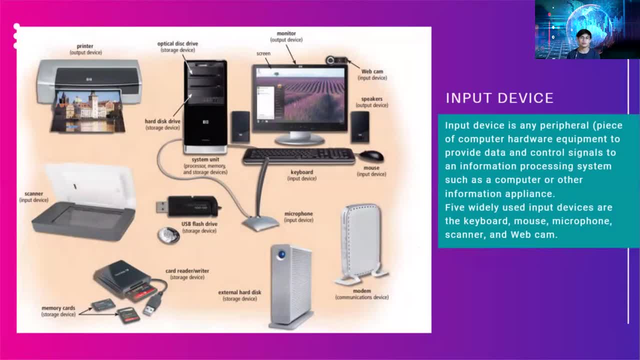 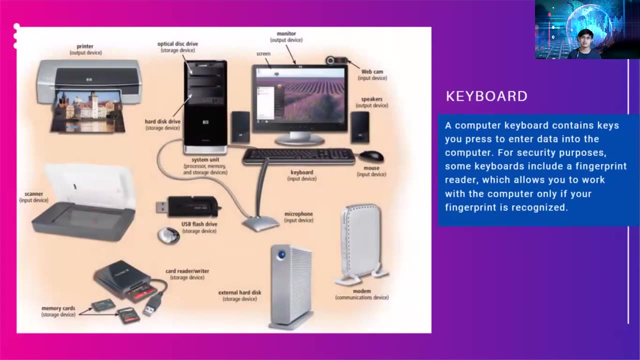 Okay, five widely used input devices are, of course, this is very known- the keyboard, the mouse, the microphone, the scanner and the webcam. So, of course, what is a keyboard? keyboard, keyboard: it contains keys to enter data into. the 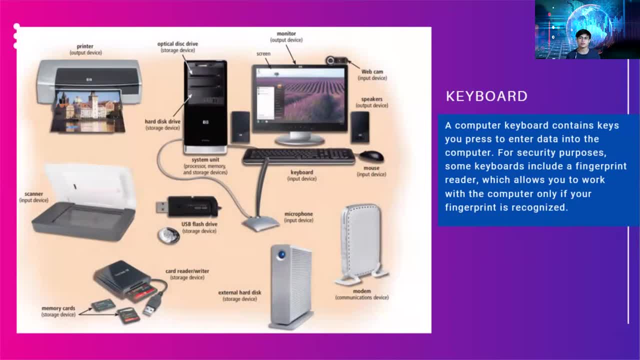 computer. for some security purposes, some keyboards include fingerprint reader, which allows you to work with the computer only if your fingerprint is recognized. so, as you can see here, yeah, that is a keyboard, so a lot of you're very familiar with it because you've been using this all the time. next we 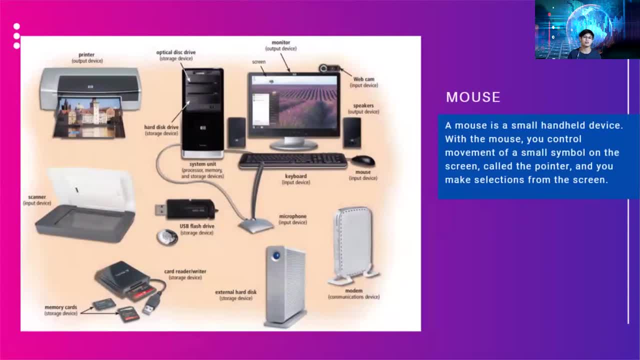 have mouse. okay, of course, the mouth is small handheld device. with the mouse you can control movement of a small symbol on the screen. okay, or call the pointer and you make selections from the screen. okay, this is the mouth. okay, this is. this is not a, an animal. I'm gonna shout mouth. okay, but I'll go the meter and you. 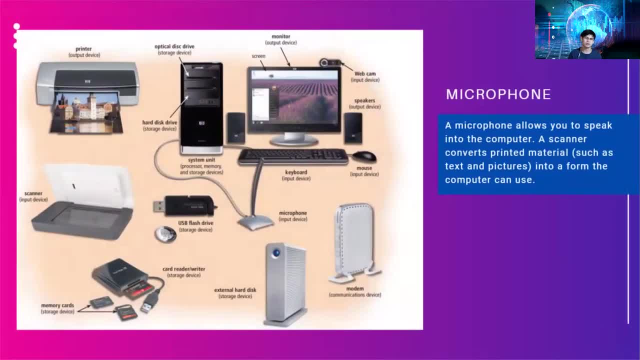 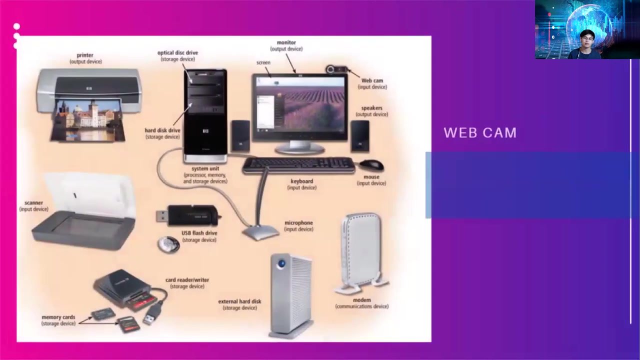 always. and then the microphone. so microphone, it allows you to speak into the computer. a scanner converts printed materials, such as text and pictures, into a form the computer can use, so it's a very you know. you know what microphone is all about. of course, a webcam or come, it's a digital video camera that allows you to 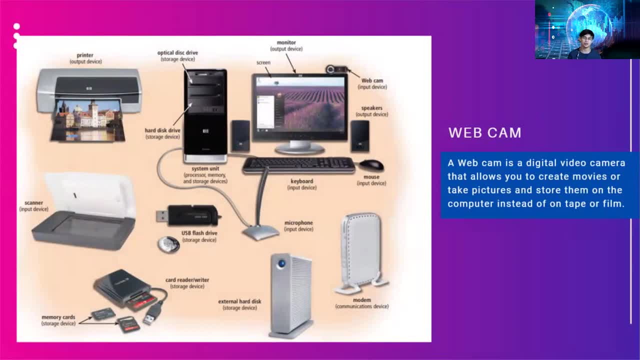 create movies or take pictures and store them on the computer. state-of-the-art or or so, though, of five most commonly used input devices. again, it includes the webcam, the keyboard mouse and, yeah, the microphone. okay, so, as you can see in the picture again, keyboard mouth, webcam, microphone. 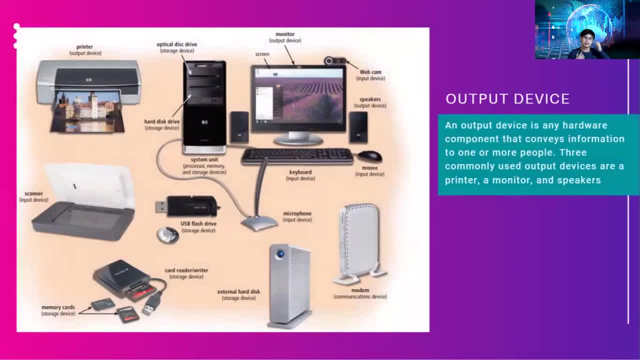 that's it next. well, we also have output devices, so this is an input, input devices. so for the output devices, it is any hybrid component that can raise information to one or more people, two to one or more people, and the three commonly used output devices are printer, a monitor and speaker. so I think we have some. point here: okay, springs and speaker. okay, so how does it look like printer and a speaker? this is specific and I think we have a sample in here. okay, so how does it look like rein DENNIS? SO I THINK IT IS ME. SO HOW DOES IT LOOK? LIKE THE EQUIPMENT? городos, or 2 minutes steps in kanai, a particular area which is in large one. okay, so people, it can change the environment according to the doctor's preferences. so are there? you make this email information about the 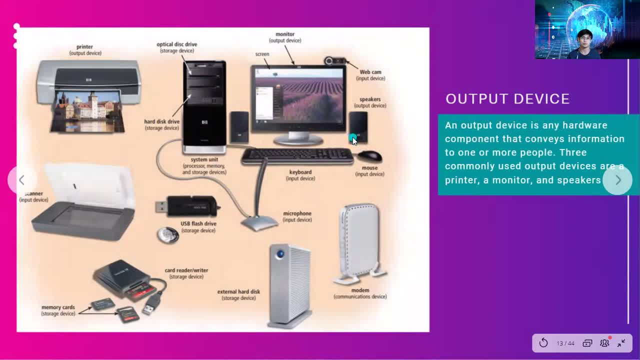 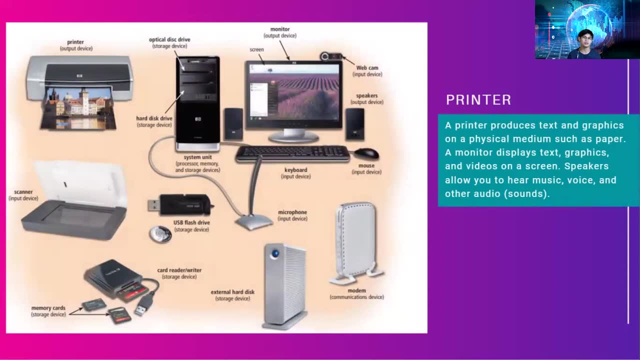 monitor and then a speaker, so those were. output device: okay, so again printer. of course it produces text and graphics and a physical medium such as paper. okay, a monitor displays a rate rate. monitor displays text, graphics and videos and screens this. speakers, allows you to hear music, voice and other audience. so yeah, 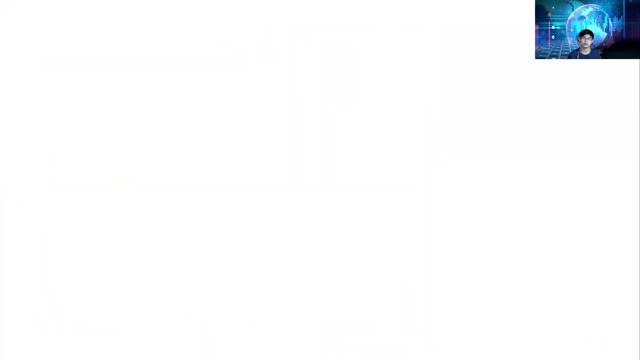 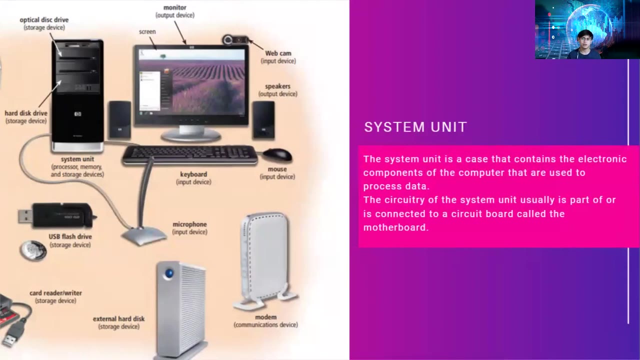 that's it. that's all for the output. right next: system unit. so what is a system unit? a system unit is a case that contains the electronic components of the computer that are used to process data. the circuitry of the system unit usually is a part of a system unit and the system unit is a part of a system unit. 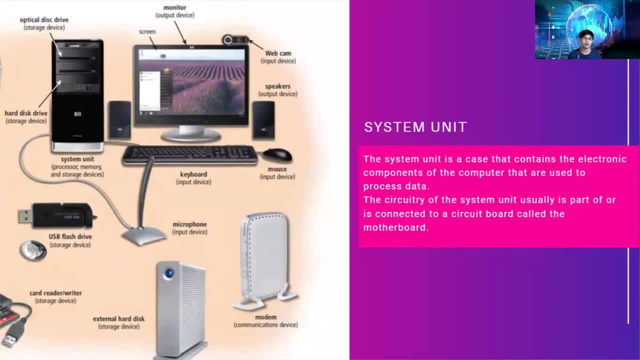 or is connected to a circuit board called the motherboard. so again, guys, this is not the cpu. a lot of you actually call this as a cpu. no, that is a system unit. okay, the cpu is just part of the motherboard. no, just part of the system unit. okay, so the system unit has the processor. 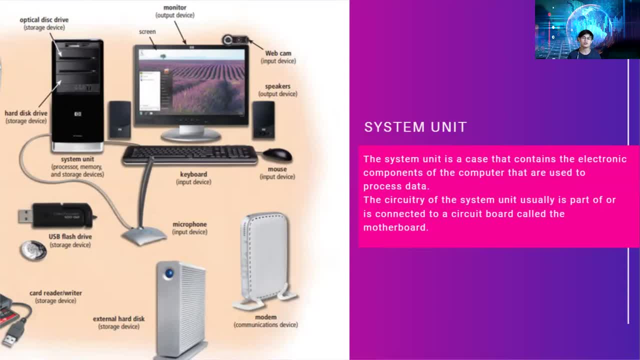 memory and storage devices. so again, that is not a cpu. a cpu is part of a system unit. so if someone asks you to please turn on the cpu, you turn on the system unit. that's the cpu. okay, so again, the system unit is a case that contains electronic components. 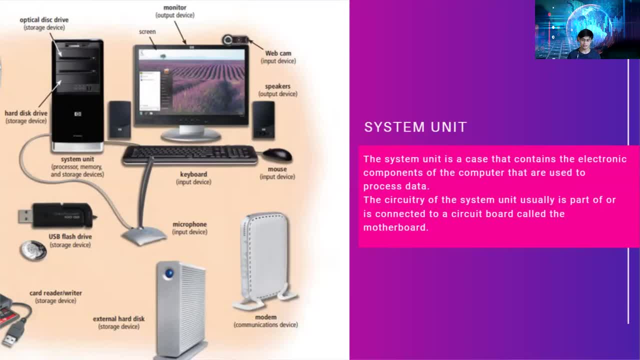 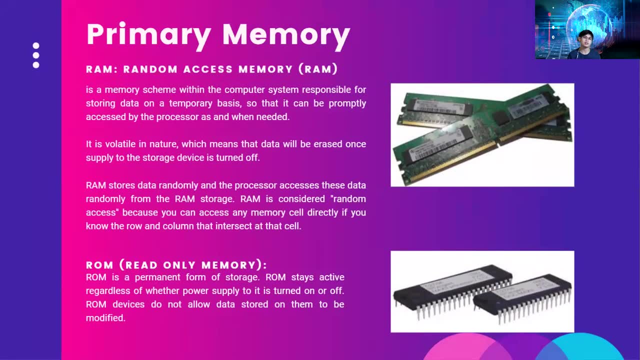 of the computer that are used to process the data. so what are the different memories? we have the primary memories and secondary memories of a computer. first memory is the random access memory or the ram. so what is the ram? ram is a memory scheme within the computer system responsible. 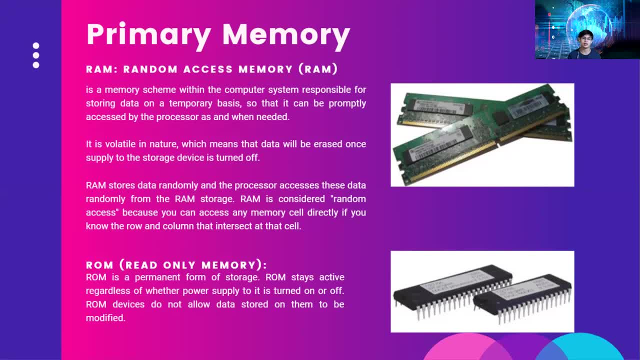 for storing data in a temporary basis, okay, so that it can be promptly accessed by the processor as when and as and when needed. so it is a volatile in nature, which means that the data will be erased once the supply to the storage device is turned off. so 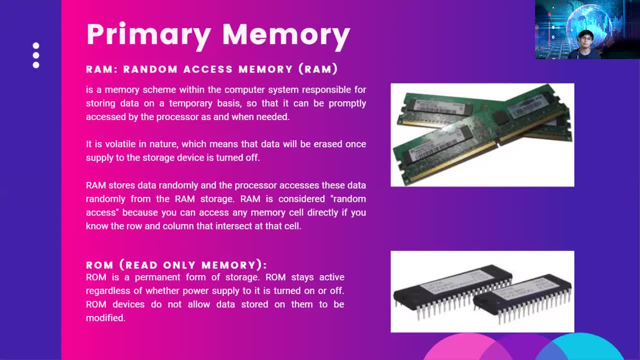 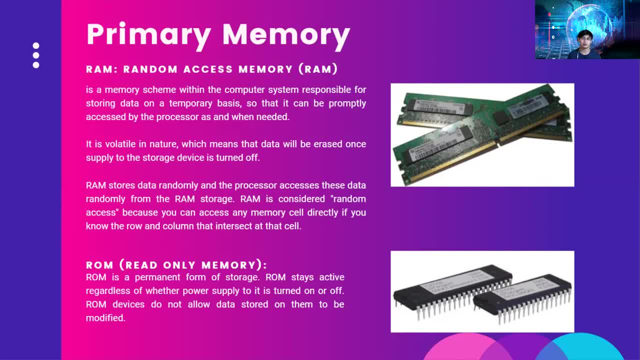 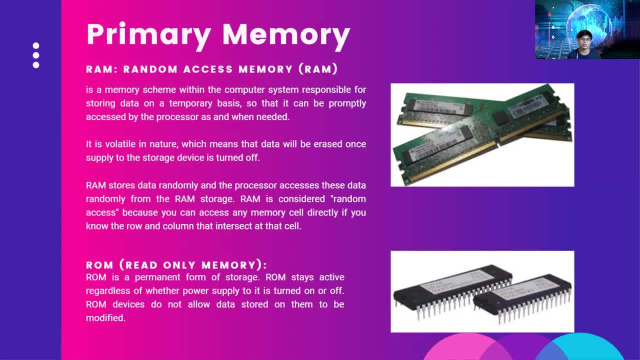 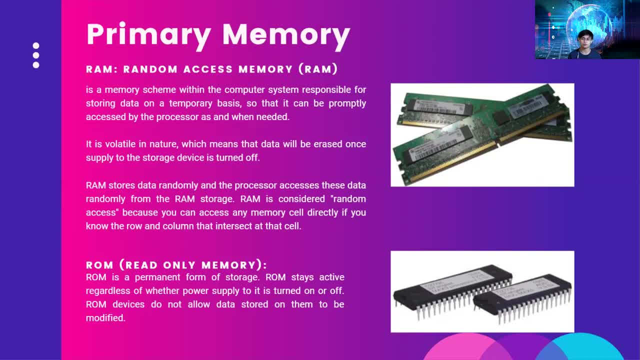 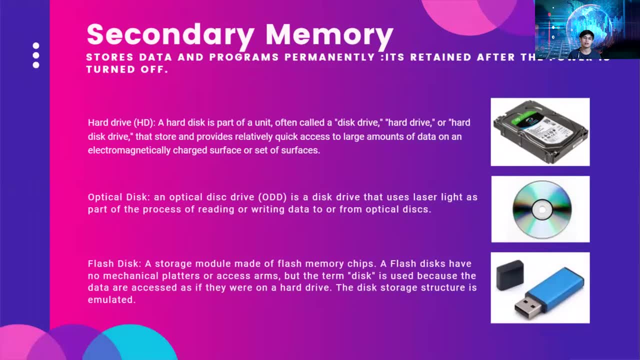 Say, room is for permanent form of storage. So I hope you understand this. Next, the secondary memory. Okay, the secondary memory, it stores data and programs permanently. okay, It retained after the power is turned off. So, even if it's turned off, 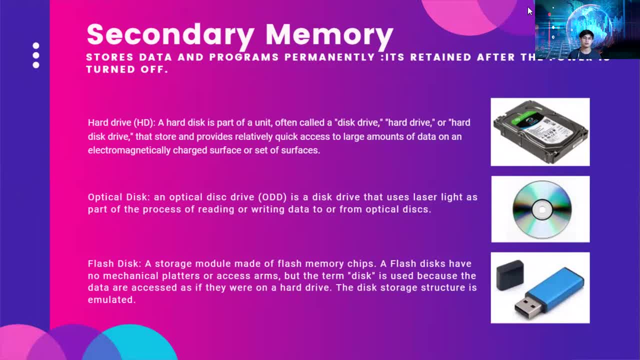 then it will. you know, the data will still remain. So first is the hard drive. okay, So what is this? hard drive or HD? A hard disk is a part of a unit called a disk drive, Hard drive or hard disk, hard drive, disk drive. 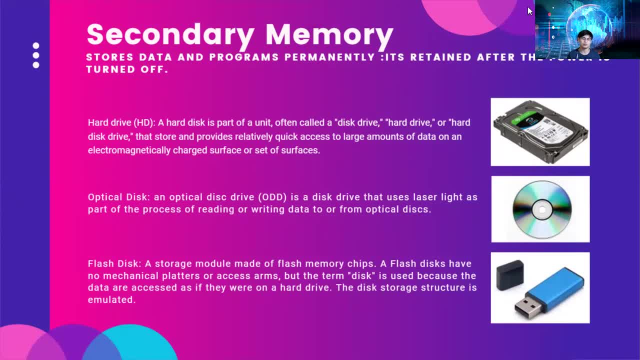 That stores and provides relatively quick access to large amounts of data on an electromagnetically charged surface or set of surfaces. So ito yung itsura niya. ganito yan, okay. And next we also have another drive, which is called the optical drive. 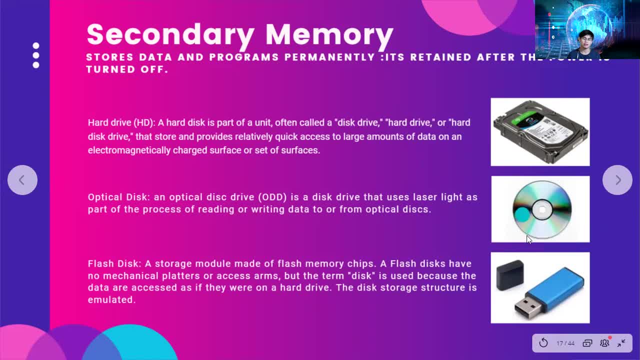 This is, I believe you always seen this: no Dago namo nakitaan ni ng mga optical disk. okay, So an optical disk drive, or ODD, is a disk drive that uses laser- Laser light- as part of the process of reading. 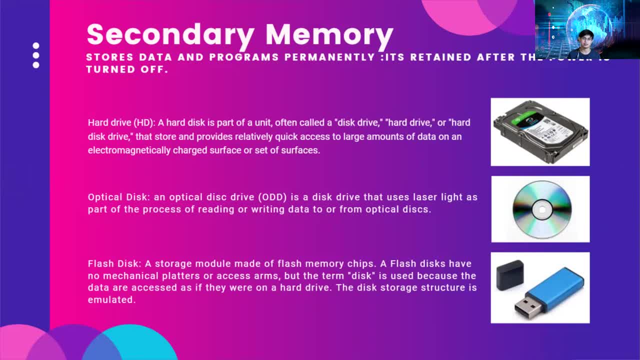 and writing to or from optical disks. okay, And then the flash disk. So this is the flash disk, dili nasa USB. okay, A lot of you call this as USB. USB is the port, universal serial bus- okay. 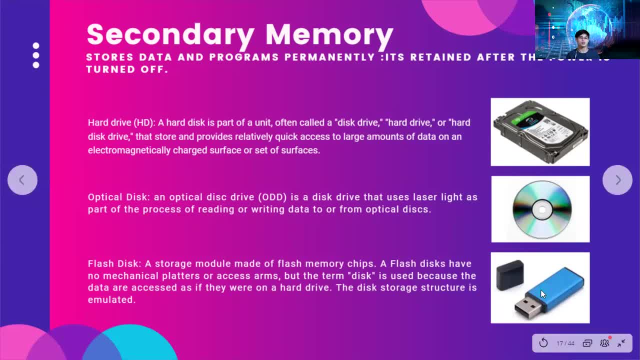 But ang tabo ginian ni is FD, a flash disk, So it is a storage module made of flash memory chips. A flash disk have a normal, no mechanical patterns or access arms, But the term disk is used because the data are accessed. 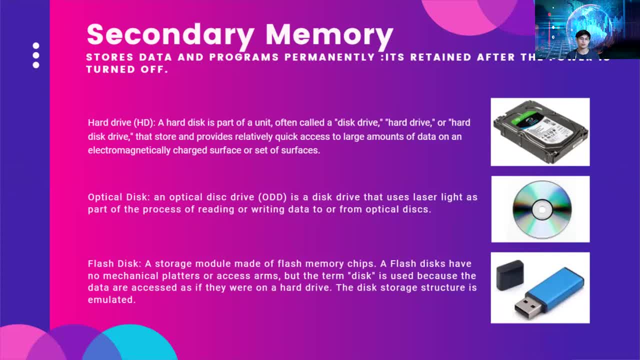 as if they were in the hard drive. The disk storage store is emulated, So I believe this secondary memories are very familiar to you guys. And nakitaan na po ito. yung niya no And nahawiran nanagamit na okay. 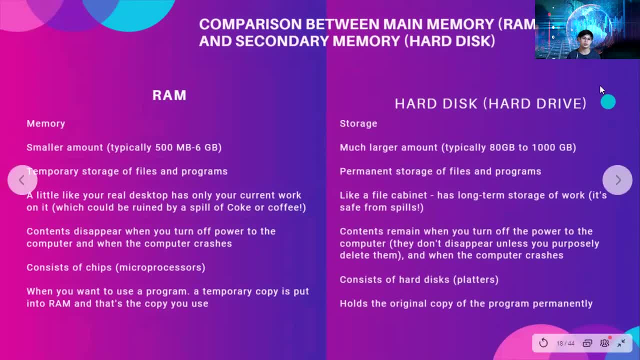 So this is the comparison between the RAM and then the secondary memory. So the RAM is the hard disk, the RAM okay. Random access memory is the memory- okay. The hard drive hard disk is the storage, The RAM smaller amount, it's typically 500 MB to six gig. 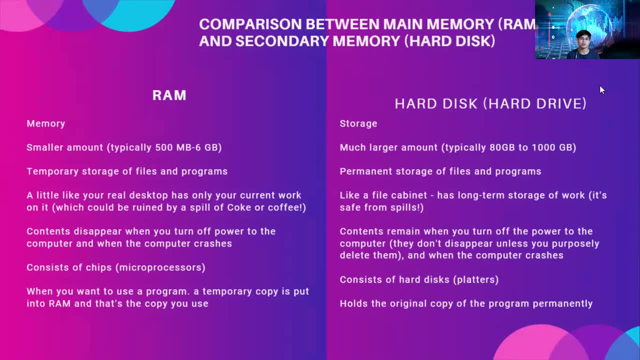 while the hard disk is typically 80 gig to 1,000 gig. okay, The RAM also is a temporary storage of files and program. The hard disk is the permanent storage of files and program, A little like your real desktop, as only your current work on it. 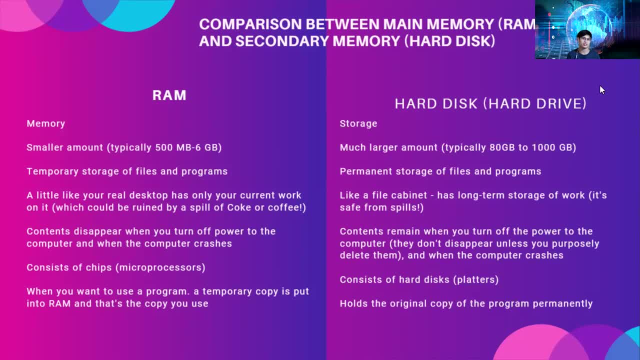 which could be ruined by a spill of coke or coffee, when it's just a RAM. But hard disk is like a file cabinet. no, It has a long-term storage of work, It's safe from spill And we also have in RAM contents disappear. 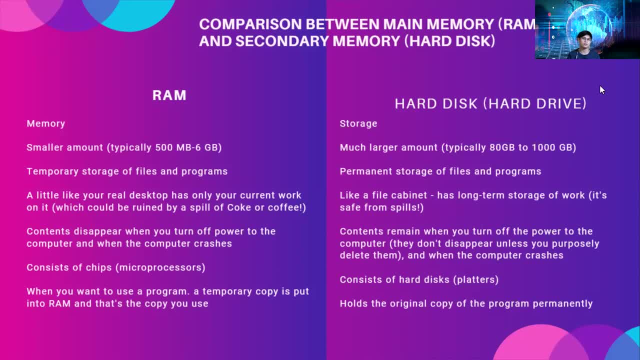 when you turn off the power, when you turn off power to the computer and when the computer crashes. But in the hard disk it's a permanent storage. okay, But in the hard disk contents remain when you turn off the power to the computer. 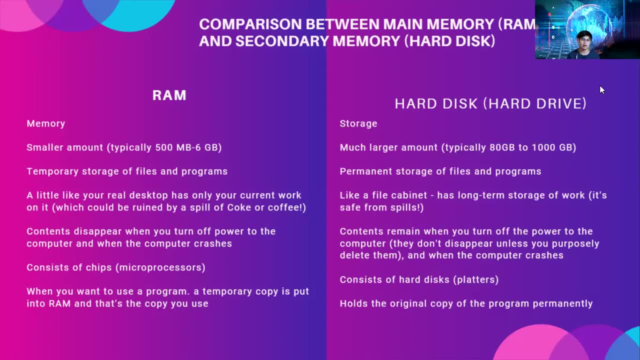 They don't disappear unless you purposely delete them. and when the computer crashes. The RAM consists of chips or microprocessor. The hard disk consists of hard disk or platters, So the RAM also. when you want to use a program, a temporary copy is put into RAM. 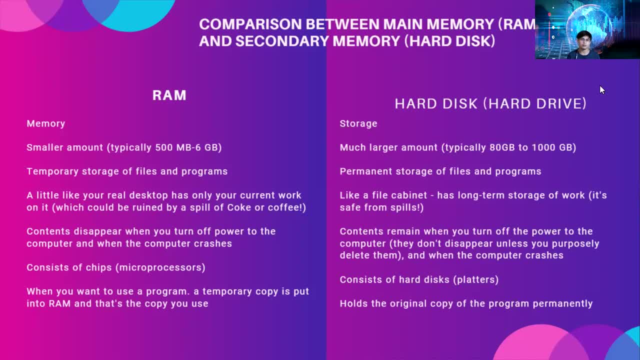 and that's the copy you use. But for the hard disk it holds the original copy, the copy of the program, permanently. So it's very important that you guys have this idea what a RAM and what is a hard disk is okay. 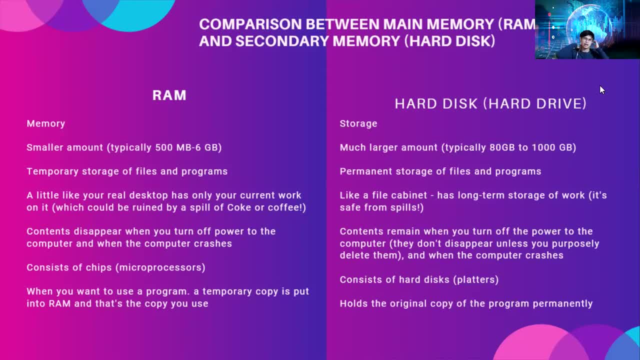 So you may have noticed, Mangod, if you buy laptops and computers that have RAMs, it's like RAM, right, It's like RAM, it's like hard disk, okay. So I hope you guys have understand now the difference between those memories, okay. 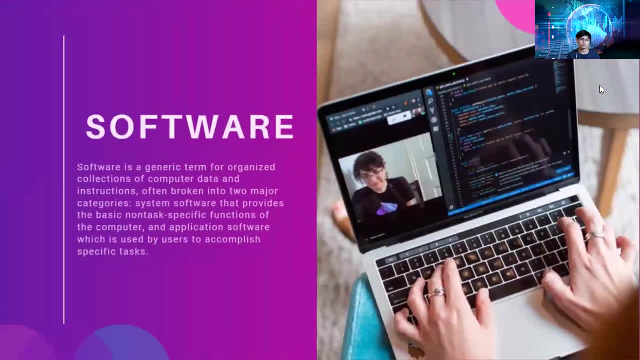 Between disk or drives. Okay, next, Next component of computer. again it's a hardware. If you haven't you know, understand anything, just you may search on it in Kogu, or you may also review this video. 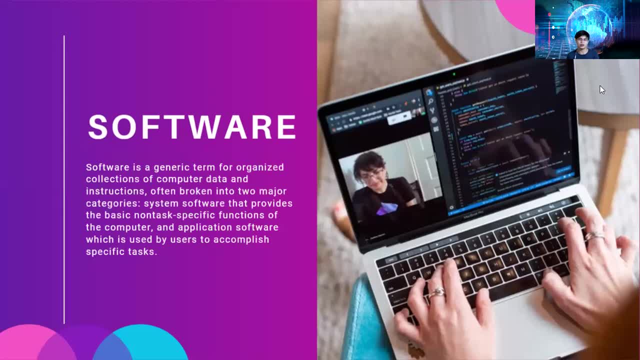 And next component of a computer is a software. So what is this software? Software is just program, right? This is a generic term for organized collection of computer data. So it's basically a system software. So the system software is a system software. 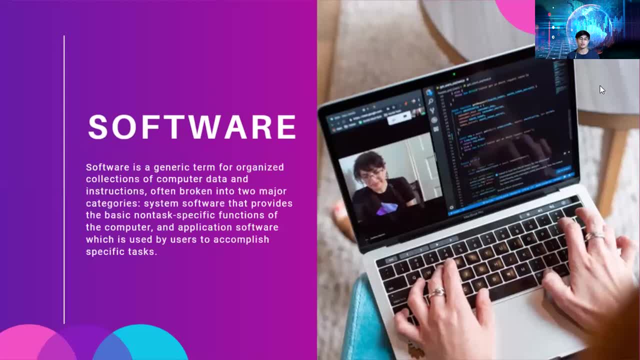 that provides computer data and instructions, often broken into two major categories: This system software and then the application software. So when we say system software, it provides the basic, NAND task, specific functions of the computer And then the application software is used by users. 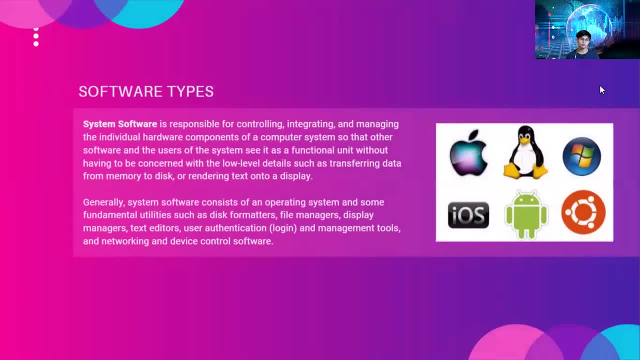 to accomplish specific tasks. okay, So again, the system software. it is responsible for controlling, you know the data. So when we say system software, it is responsible for controlling and degrading and managing the individual hardware components of a computer system so that other software 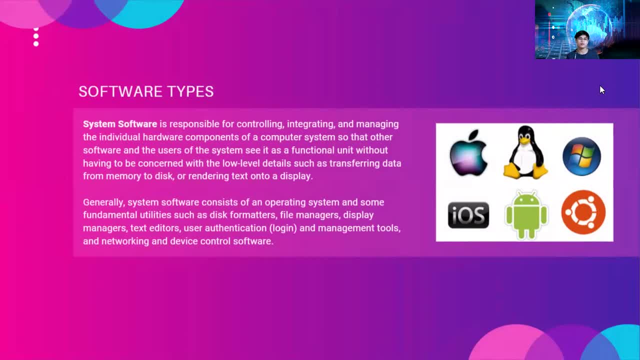 and users of the system see it as a functional unit, without having to be concerned with the low level data such as transferring data from the memory to disk or rendering text into display. And generally, system software consists of an operating system. I believe you are very familiar with operating systems. 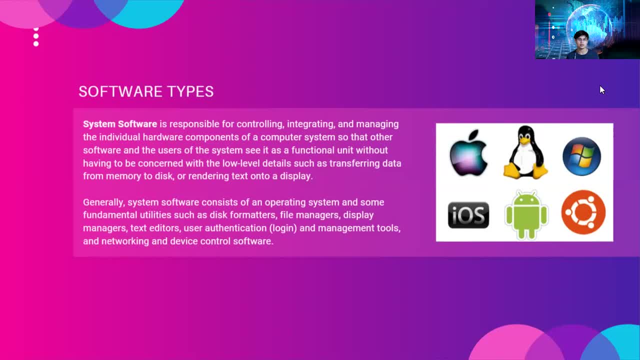 and some fundamental utilities such as disk formatters, file managers, display managers, text editors, user authentication and management tools and networking and device control software. So again, I know that you are familiar with Windows, Linux, iOS, Android OS, something like those things. 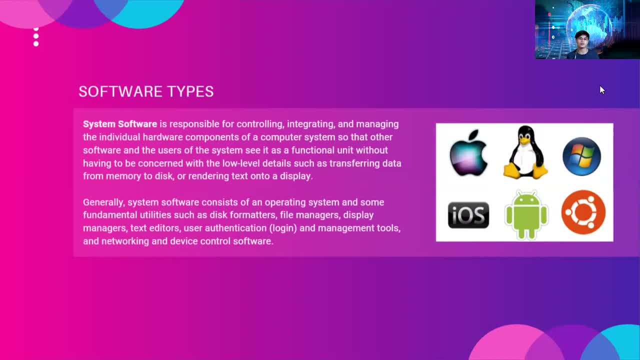 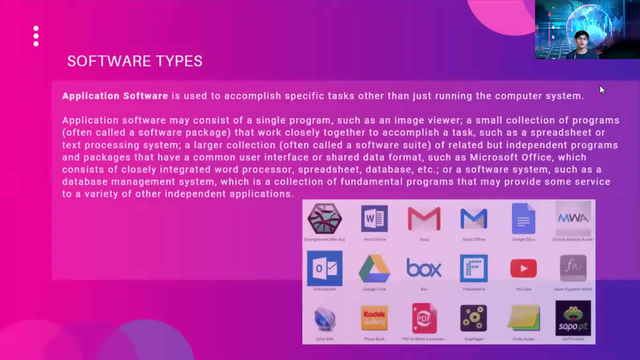 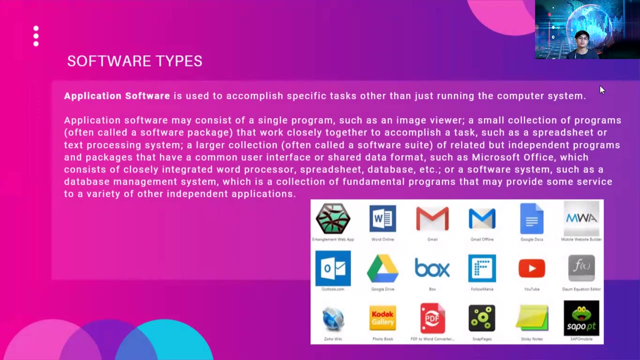 So I'm going to show you the system software. Okay, So I'm not sure what they call it. Okay, And we also have application software. The application software is used to accomplish specific tasks other than just running the computer system. Okay, 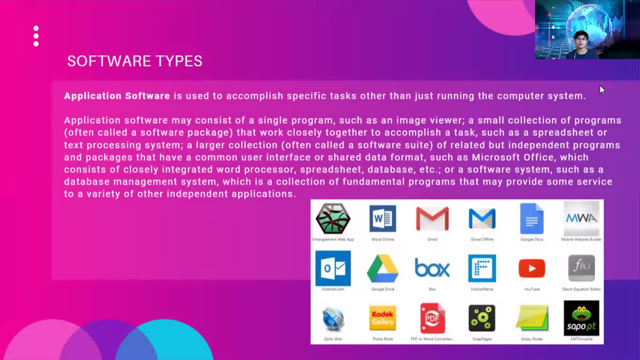 It consists of a single program. Again, it consists of a single program. Example: an image file, An image viewer, A small collection of programs, or often called as a software package, that work closely together to accomplish a task such as you know, we have a spreadsheet. 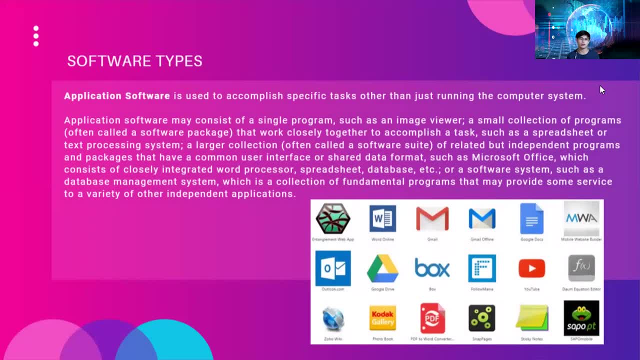 text processing system, or it is also called a larger collection or the software suite to related but independent programs and packages that have a common user interface or shared data format. Okay, We have some examples: Microsoft Office, which consists of the integrated word processor. 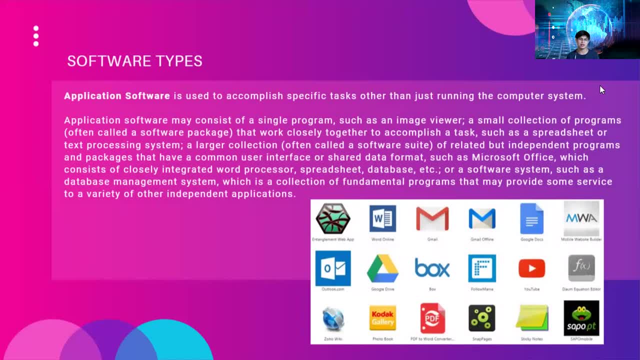 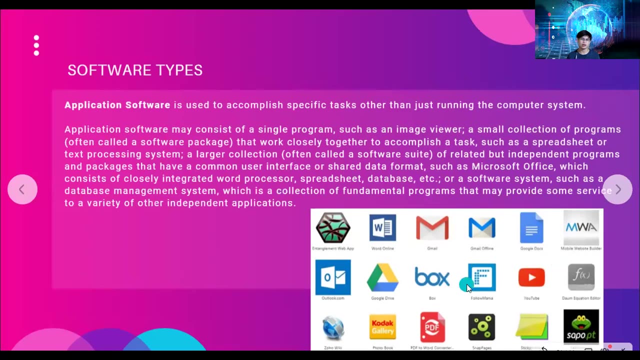 spreadsheets, databases, et cetera. Okay, And also it is a collection of fundamental programs that may provide some service to a variety of other independent applications. So, as you can see, we have sample applications here: Google Drive, Gmail, Word, et cetera. 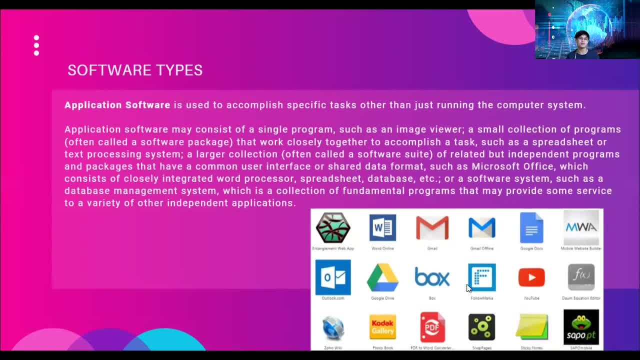 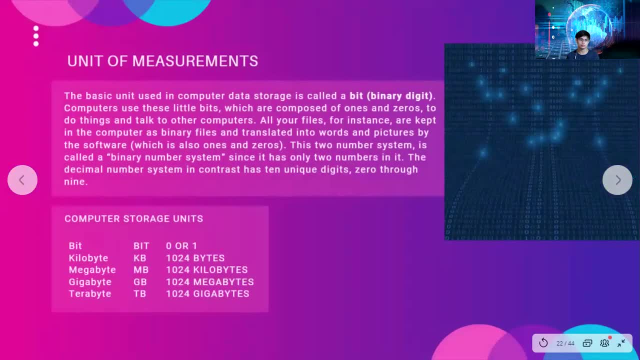 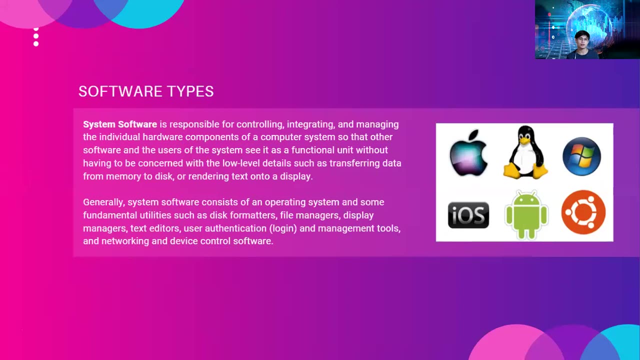 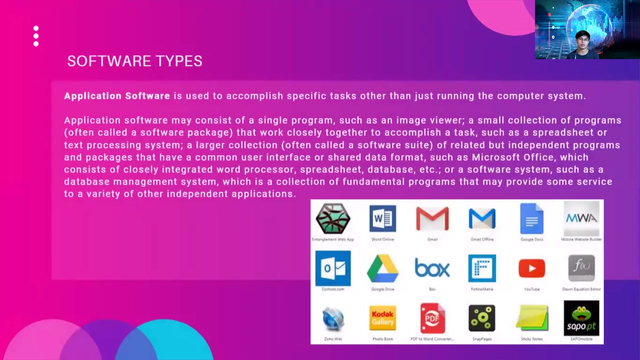 I'm going to install this. I'm going to install this in the computer. Okay, So the comparison. Okay So again, the system software. it is responsible for all the controlling, integrating and managing the individual hardware components. The application software is the program. 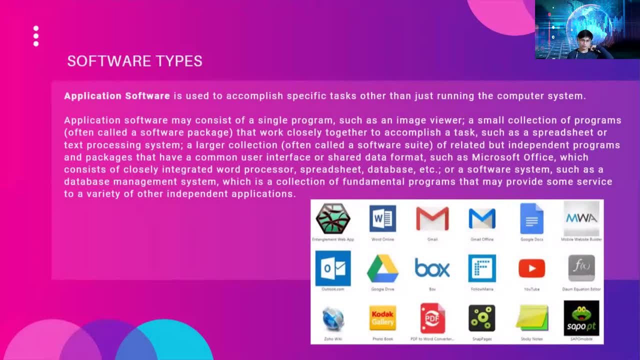 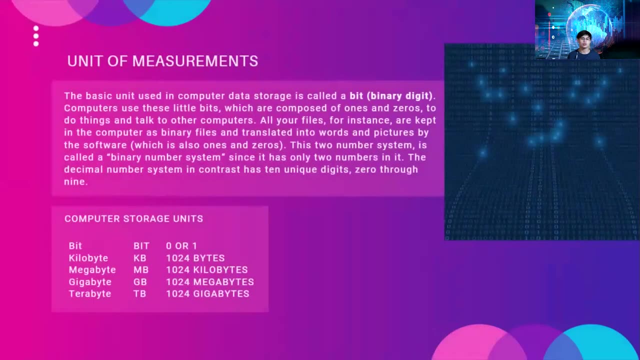 It is just a single program. Okay, So you guys have understand the comparison between the application software and then the system software, So let's move on with the unit of measurement. So it's very important also that when studying the basic components of the computers, 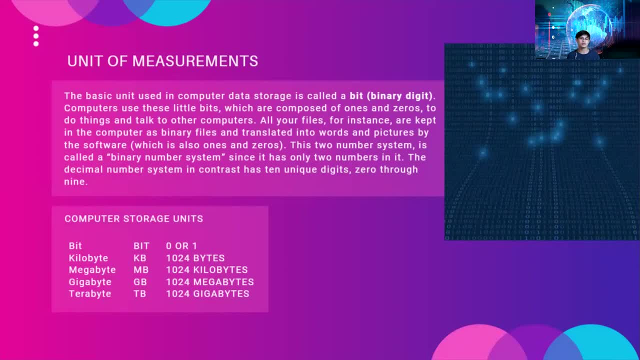 you know the unit of measurement. So the basic unit used in a computer data storage is called a bit. Again, the basic unit used in a computer data storage is a bit or binary digit. So what is this binary digit? The one and zero. 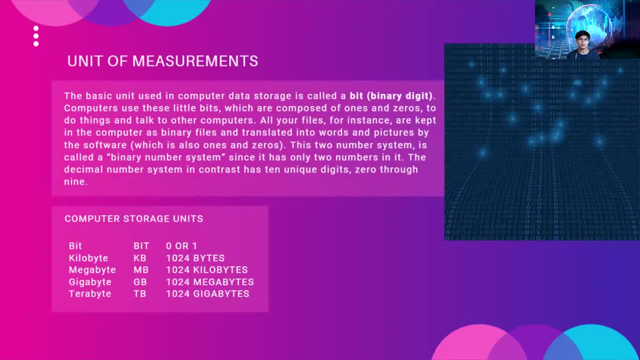 So I know, guys, that you're not yet very familiar with this, but don't worry, because in the next chapters we will be Okay. So computers use these little bits, which are composed of ones and zeros, To do things and talk to computers. 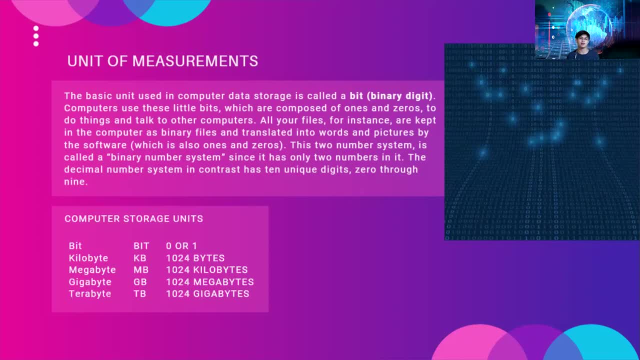 Okay. So when you actually provide inputs to your computer, it will be processed And by processing that the computer translates it to its computer language. to you know, binary digits to one and zero. Okay, To do things and talk to other computers. 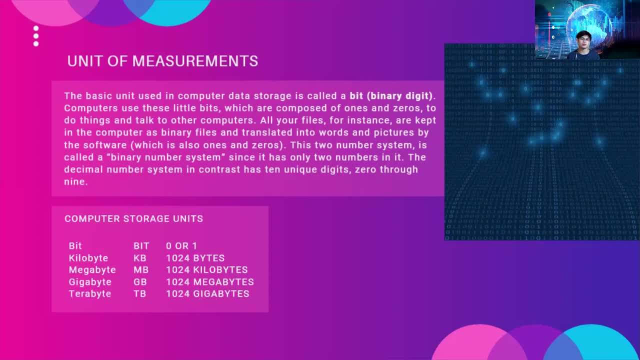 So all your files, for instance, are kept in the computer as a binary file and translated into words and pictures by the software, which is also ones and zeros. So this two-number system is called a binary number system, since it has only two numbers in it. 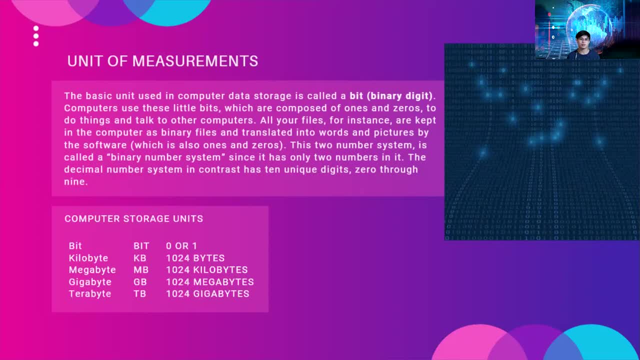 Okay. Binary- The decimal number system is contrast- has ten unique digits, Zero to nine. Okay, So we have this sample Computer storage unit, bit one, bit zero or one. The kilobyte or the KB is actually around 10,024 bytes. 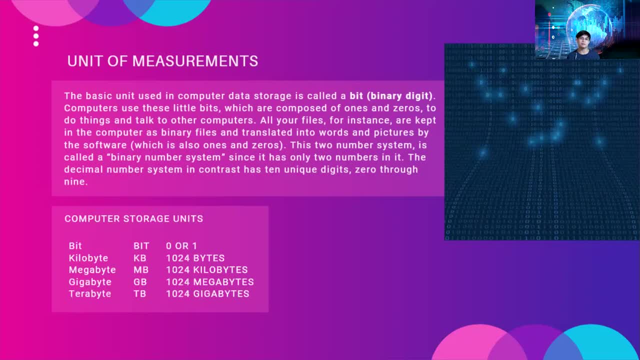 Okay, The megabyte, or MB, is 10,024.. 1,024 kilobytes. Sorry, the kilobyte is 1,024 bytes. Okay, The megabyte is 1,024 kilobytes. The gigabyte is 1,024 megabytes. 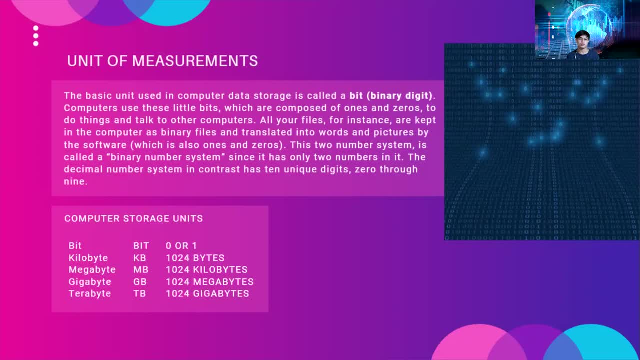 The terabyte is 1,024 gigabytes or the TB. So I hope you familiarize yourself with the different computer storage units that are used in the computer. So again we have bit, kilobyte, megabyte, gigabyte. 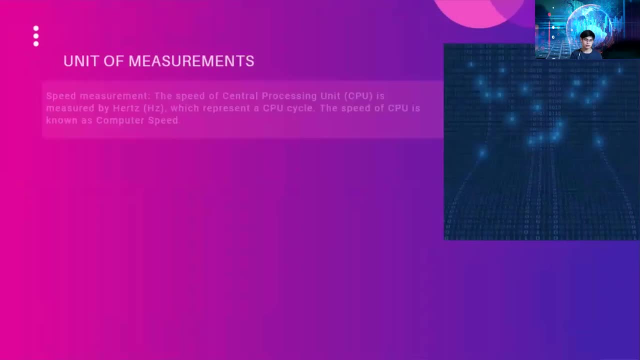 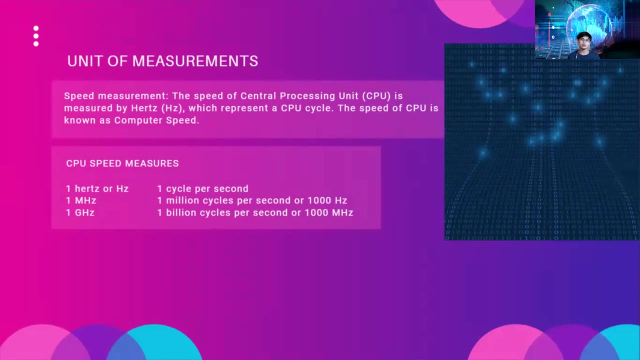 or terabyte. Okay, So next is the speed measurement. So the speed of central processing unit or the CPU is measured by hertz, HZ. Okay, Again the speed of a central processing unit or the CPU. Again, the CPU is part of a system unit. 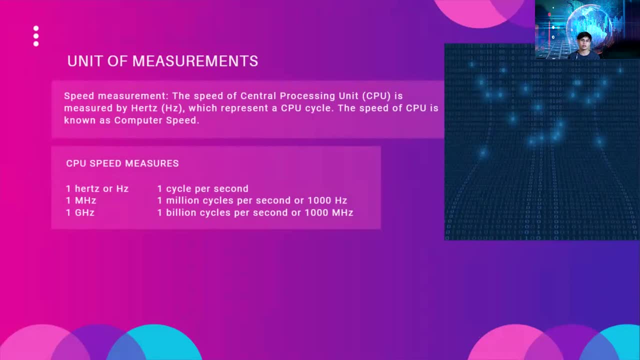 which is measured by hertz. Hertz, Okay. So which represents a CPU cycle. So the speed of a CPU is known as computer speed. Okay, The CPU speed measures are as follows: One hertz or HZ. one cycle per second. 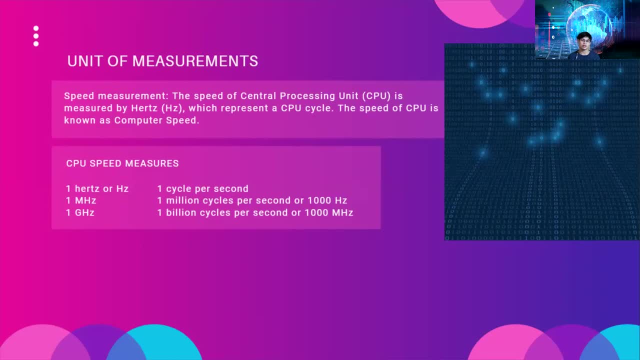 Okay, And one MHZ is one million cycles per second or 1,000 hertz, And then the one GHZ is one billion cycles per second or 1,000 megahertz. Okay, So that is gigahertz. 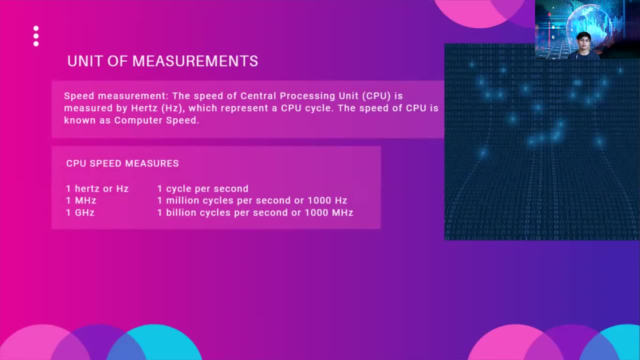 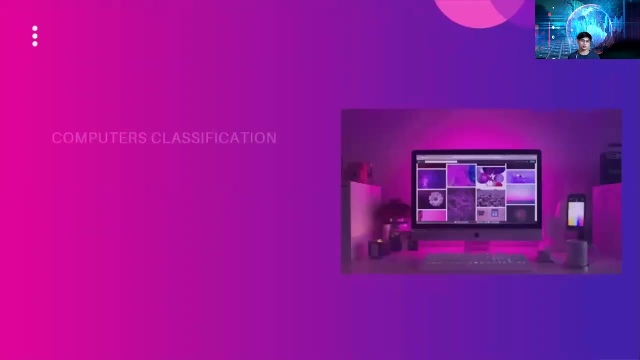 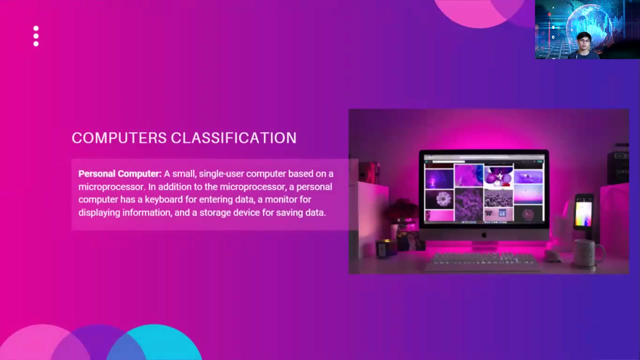 and then megahertz. Okay, So please familiarize yourself with the speed measurement also. Next, the computer classifications. So I hope I believe this is very, you know, pretty basic and we have been using this all the time. 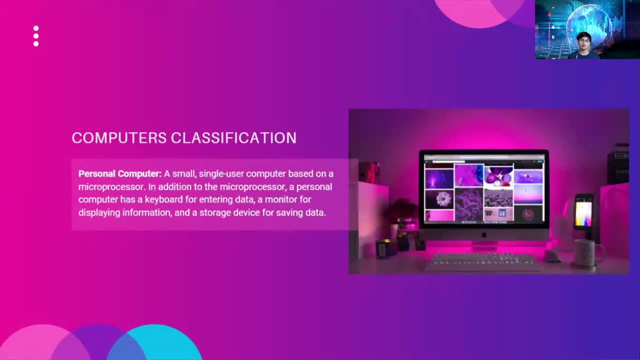 So we have first the personal computer. Okay, Personal computer, A small, single user computer based on a microprocessor. So, in addition to the microprocessor, a personal computer. of course. it has keyboard, it has monitor and the storage device for this, for savings. 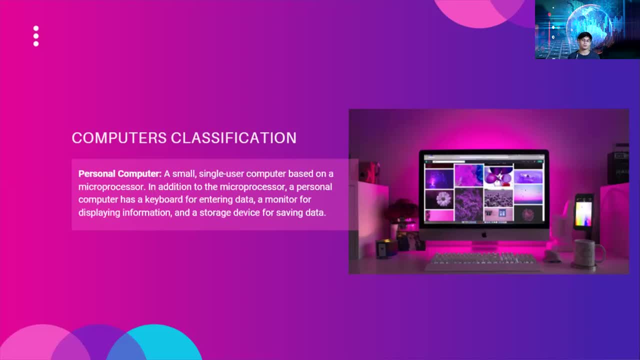 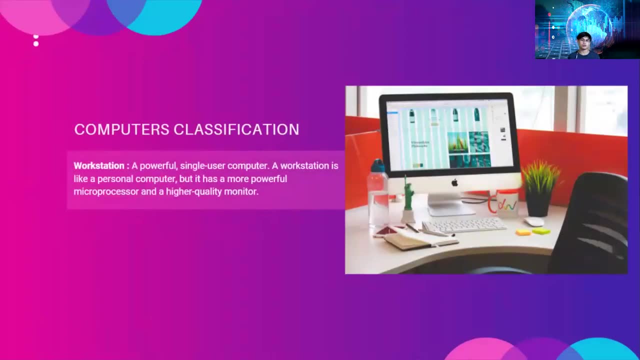 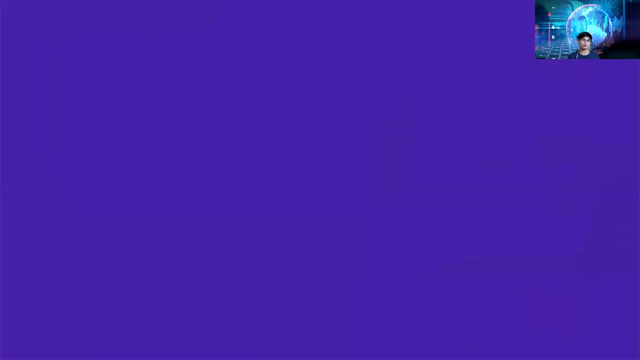 okay, so because i gotta figure this in your head on has a personal computer, or yeah, and of course workstation. so in a workstation there's a powerful, single, single user computer. it is like a personal computer but it is more powerful: microprocessor and higher quality monitor. so middle, high end, of course it's for work, okay. and then the mini. 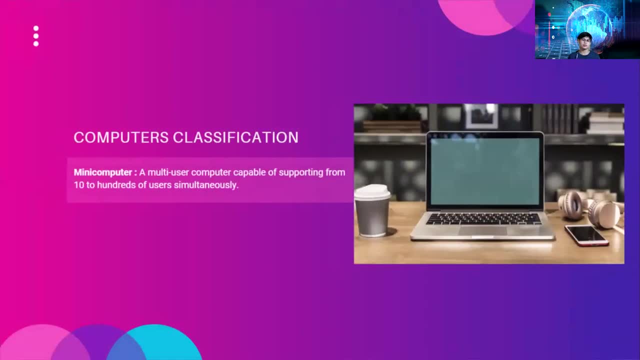 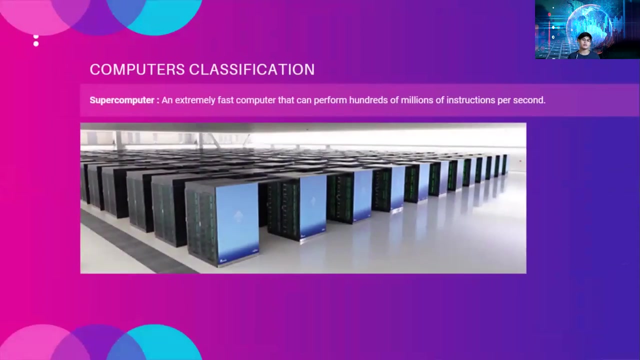 computer. uh, the mini computer is a multi-user computer. it is capable of supporting from 10 to 100 users simultaneously. so this is actually not the image, this is just a sample image. and next we have the supercomputer: the super computer, An extremely fast computer that can perform hundreds of millions of instructions per second. 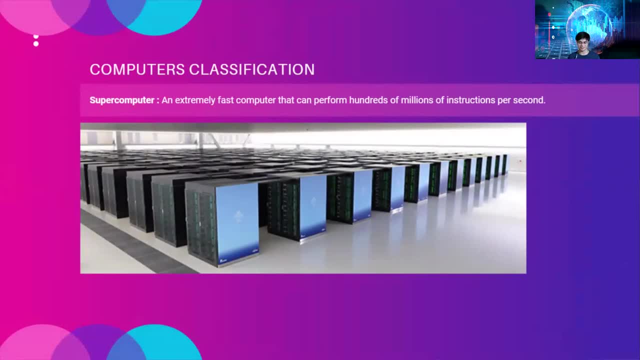 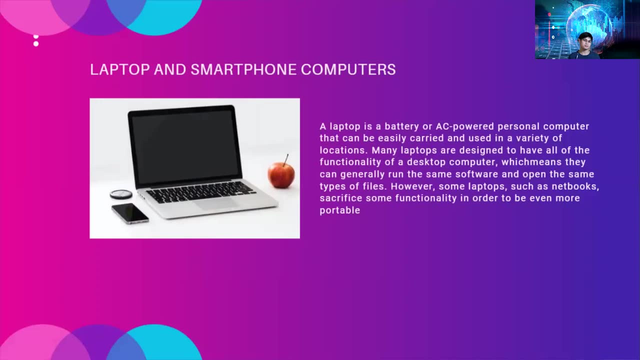 So do you have a support computer in there? It's really awesome. Okay, next is a laptop. laptop Very familiar with you guys. I can't believe I used money. I can see you. Is it is a battery or is it our personal computer that can be easily carried and used in a variety of locations? 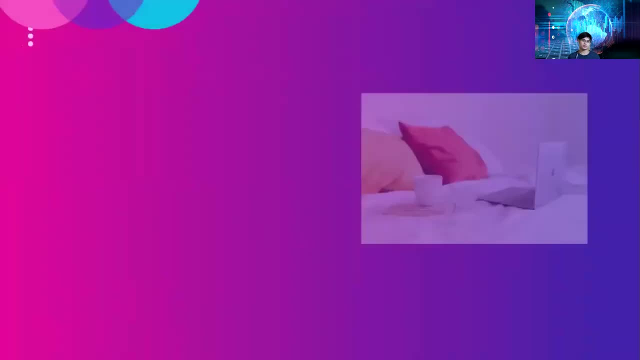 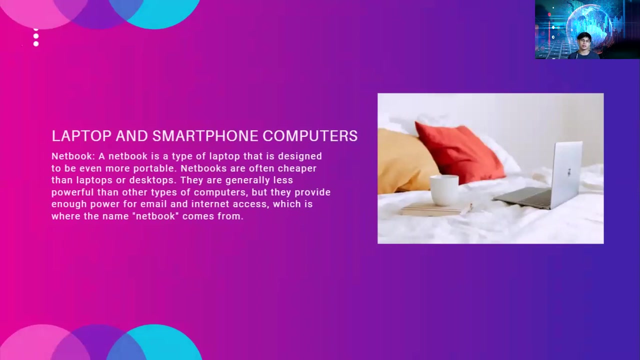 Okay, So the unit I know to share the guy- you know, it's a balloon, Amanda course- netbook is. This is a kind of a type of laptop that is designed to be even more portable. Then we do the mega misha. Okay, these are often cheaper than laptops or desktops. So 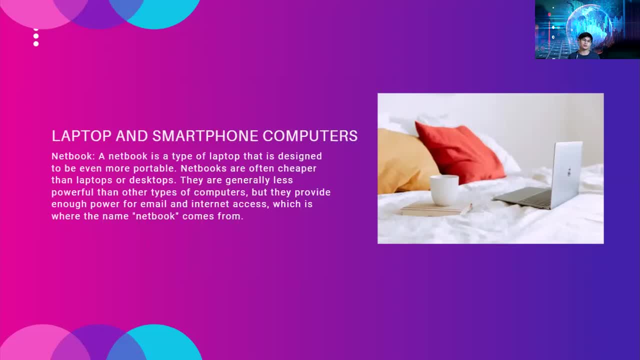 These are general, generally less powerful than other types of computers, But they provide enough power to email and internet access, which is where the name it book came from. So if you're, if you're just using it for online classes or just simple onion button, simple and buttons is a computer, then a netbook will do okay. but I'll come and check a. 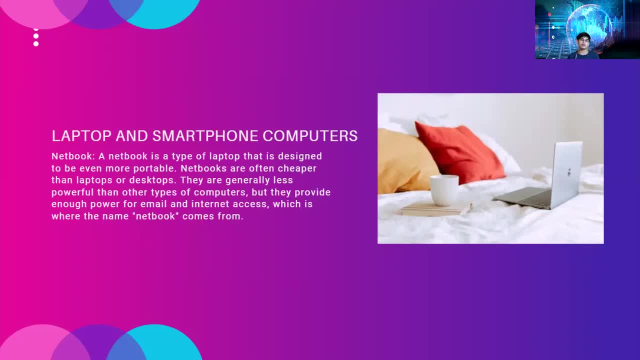 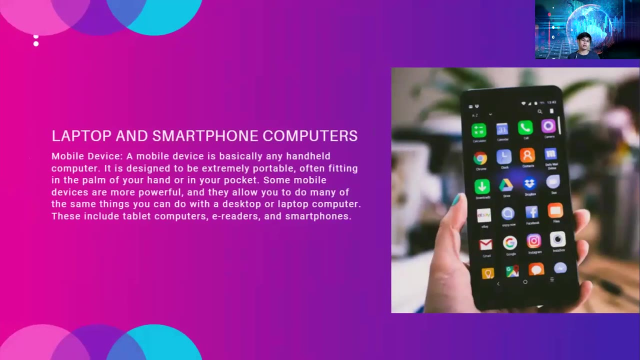 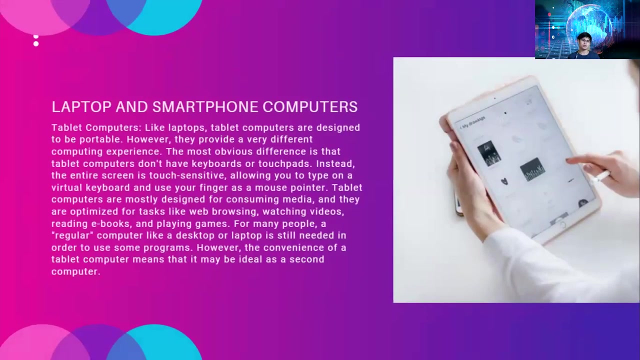 laptop, pero sacaron, I think Net book and laptops, and we're preparing the channel price So better and along by with laptop, Okay, of course. mobile device, no, smartphone. tablet, Okay, Tablet, of course you. you know what the tablet is? No, it is like a laptop, It is designed to be. 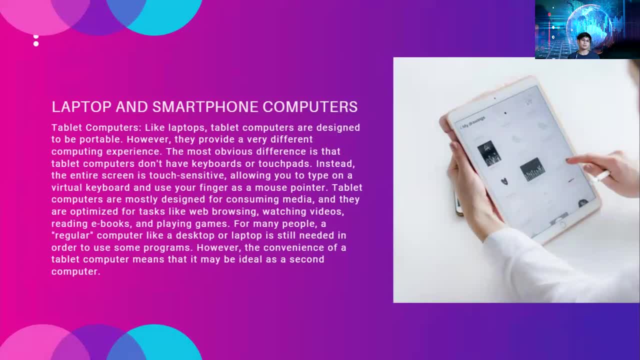 more portable. so it has. it Provides a very different computing experience. But there are actually tablets today now. but you know, say if that's pretty, come hot at your keyboard, and mom, But I'm a bun, It's a lot Okay. So I hope now cabrón amana. 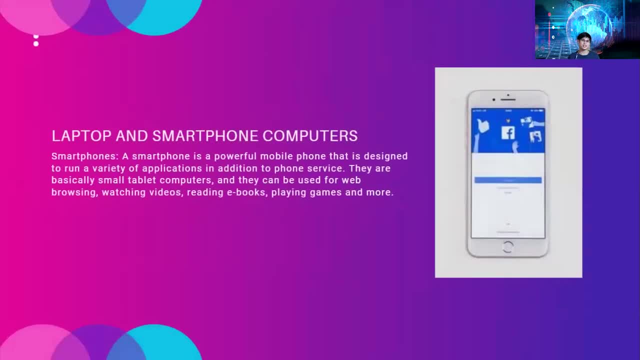 And I know none of them attain you. and then Kenny, I believe everyone has smartphones, Okay. so smartphone, It is a powerful mobile phone that's designed to run a by variety of applications In addition to the phone service. So, currently, below in your online flexible learning, I believe you're using your smartphones right. 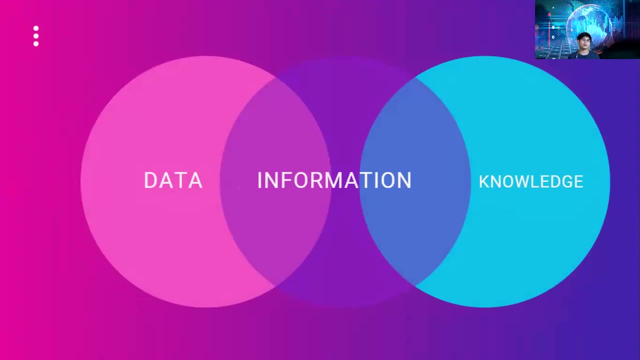 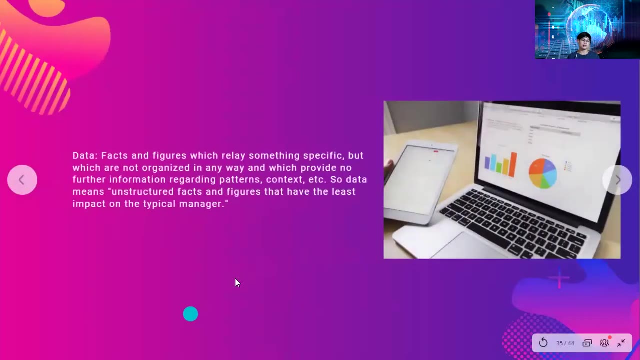 Okay, now let's move forward and differentiate. what data? what is the data? information and knowledge. So when you say data, Data are the facts and figures which really something is specific, But which are not organized in any way and which provide no further info of information regarding patterns. 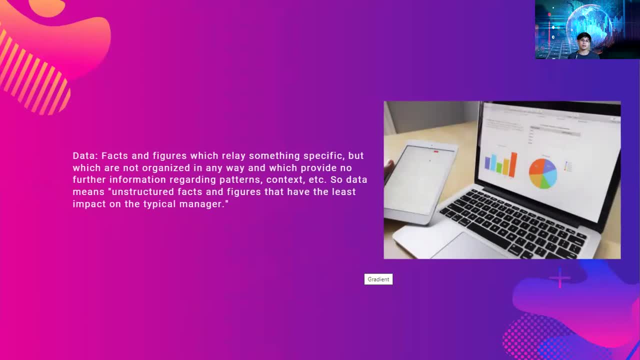 context or etc. So data means unstructured facts and figures that have the least impact on the typical integer. Again, these are just the facts and figures, which really something specific is. for example, You wanted to count how many, How many, How many born males and females for the year 2020. so what you're going to do is you are just you know, find a date on it. 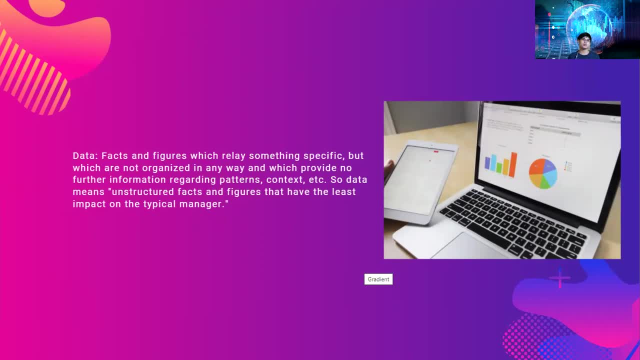 No, you check home, You just check, You know. just a piece of Information. guess the deletion information. Okay, more of a shag. More figures, okay, More. More of a passion. organized the man, Anubha the man. so For me you're able to secure one, okay. 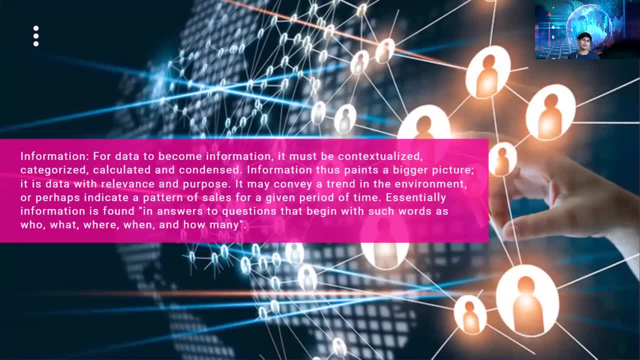 Next information or information. for data to become information, It must be contextualized. So if you wanna get the more data that when textualize anymore, then that is the information. It's already categorized, It is calculated and condensed, so information does paints a bigger picture. so it is data with relevance and 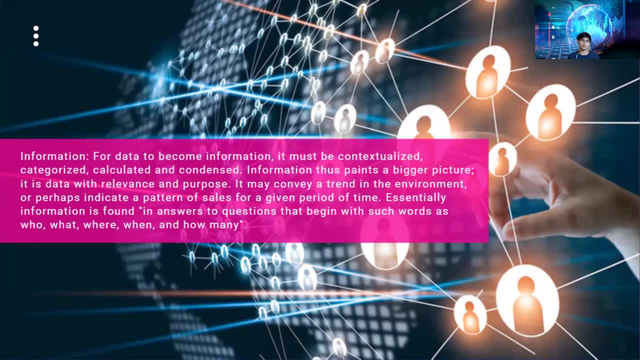 purpose. it may convey a trend in the environment or perhaps indicate a pattern of sales for a given period of time. Essentially, information is found in answers to questions that begin with just word as who, what, where, when and how many. so again, When the data is contextualized and categorized, 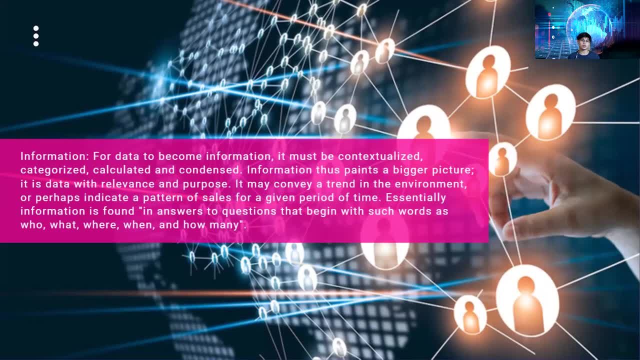 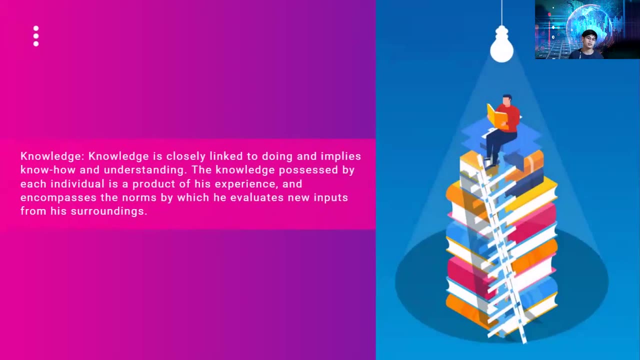 It could be. it is called the information. So again, the information paints bigger picture. Then the knowledge. the knowledge is closely linked to doing and implies know-how and understanding. the knowledge possessed by each individual is a product of his and encompasses the norms by which he evaluates new inputs from his. 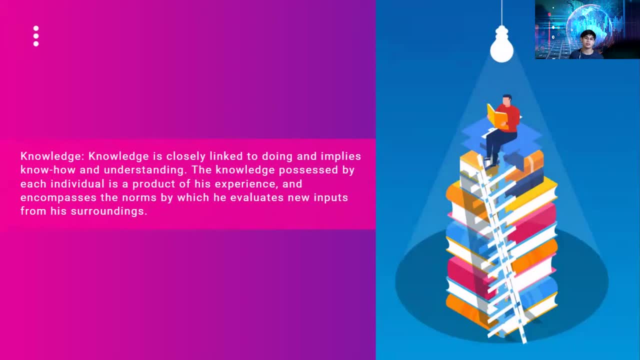 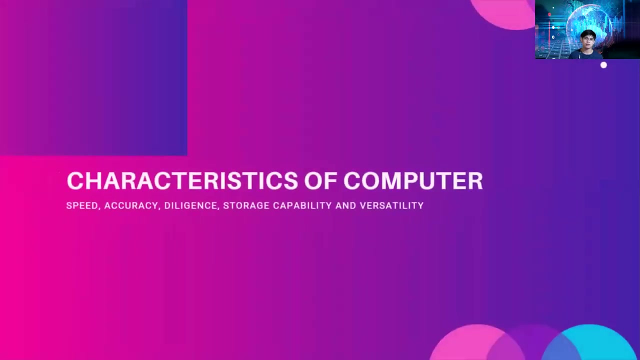 surroundings. these are the learnings that you get. okay, again, it's linked to doing and advice, know-how and understanding. okay, so so I hope that. why? why we did discuss the data, information and knowledge, because it's very important that you know those terms, because that is what the computer do. no, 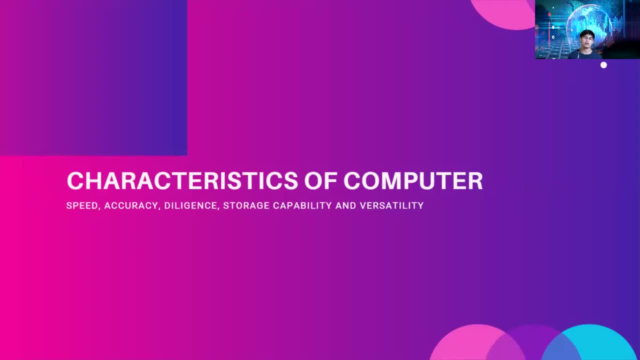 you give data, it for the same, for it's being processed, and it gives you information and then you get the knowledge. okay, so let's discuss the characteristics of a computer. of course, a computer has a speed, curacy, diligence, storage capability and personality, so there are a lot of things that you can do. 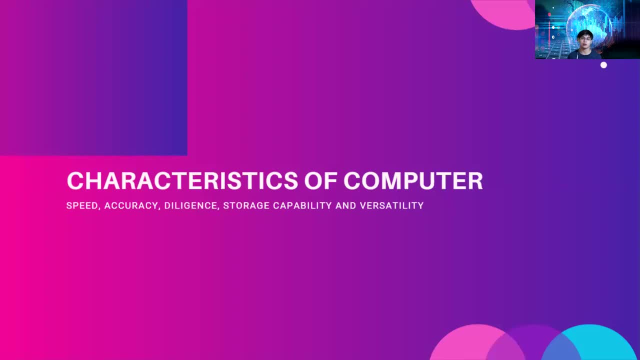 with computers, and especially today that we are in a flexible learning. so it would be very hard to do this through this online learning if we don't have computers. so imagine how are we going to do it, okay, okay, so let's talk. no man with different computer viruses. 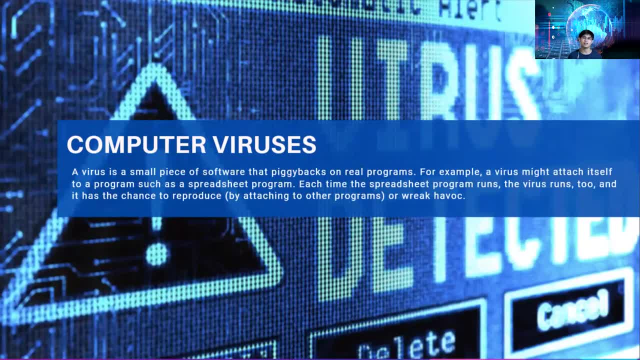 so of course there are virus, you know, just like human being, ama, vital sign, the computers, also pretty similar by Assam. okay, so a virus is a small piece of software that piggybacks and real programs. okay, so, for example, a virus might attack itself to a program such as a spreadsheet program. so each time the 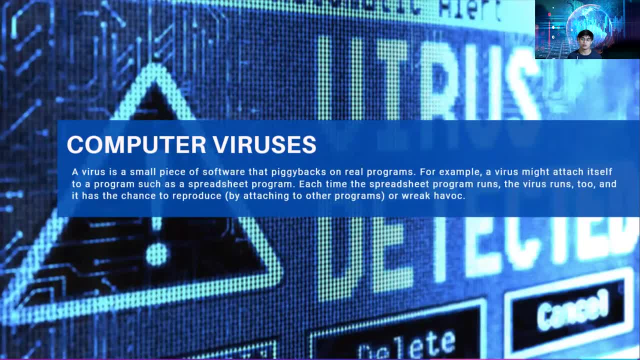 spreadsheet program ones the virus runs runs to and it has the chance to reproduce by atta or wreak havoc. So it's possible that the different applications will get crashed, Or it's possible that the virus can damage your computer. It will block your blue screen. 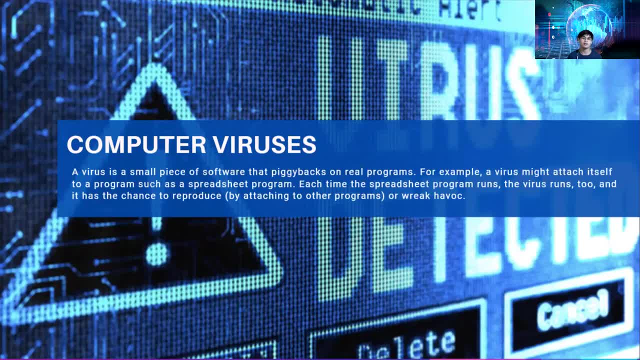 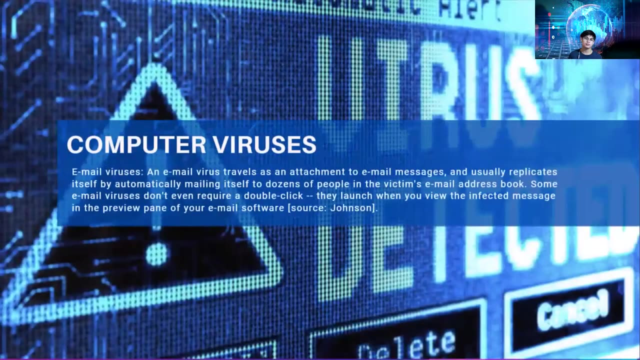 You'll just have to use your hard drive. So it's very important that you familiarize yourself with the different viruses. What are the possible viruses that you can attack on your computer? First, we have email viruses. As for the email viruses, an email virus travels as an attachment to email messages. 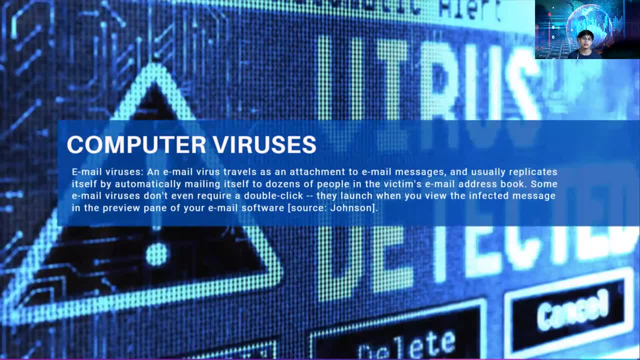 And usually replicates itself by automatically mailing itself to dozens of people in the victim's email address book. Some email viruses don't even require a double click, So they launch when you click. You view the infected message in the preview pane of your email software. 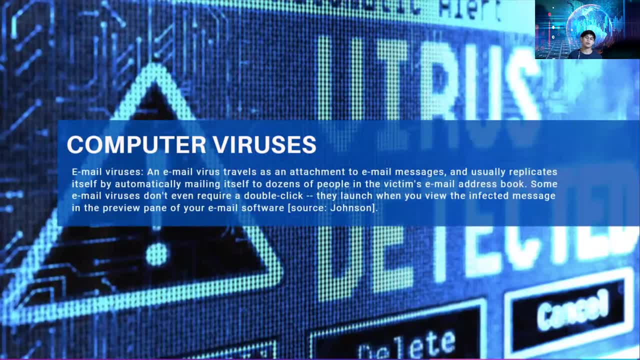 So it's very important, guys, that if you You know it's not enough to just subscribe to any other websites to get an email, Okay, you must also protect your emails And do not just click anything where they send your email. 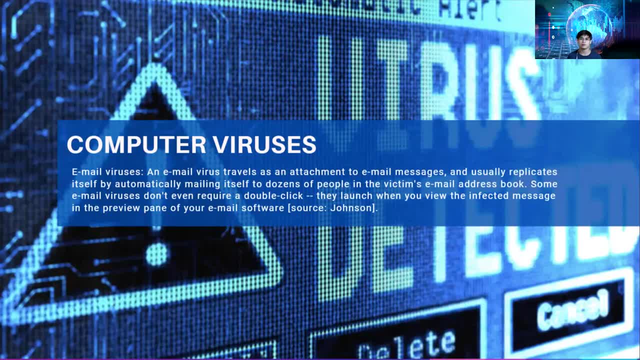 It should be legit. You should be able to see if it's spam. So meaning really, If it's a spam message, just don't open it, Just delete it, Okay. So it's very important that you don't just simply click it. 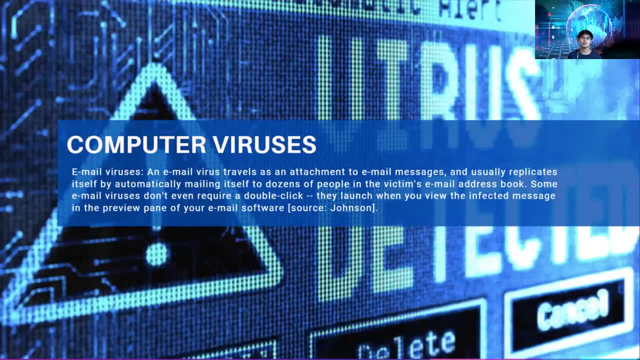 If you feel like it's a fake email, then don't click it. Okay, It's the same for those who have 1 million followers, Those who have phones, iPhones and other emails. So it's clear to you that those were not legit emails. 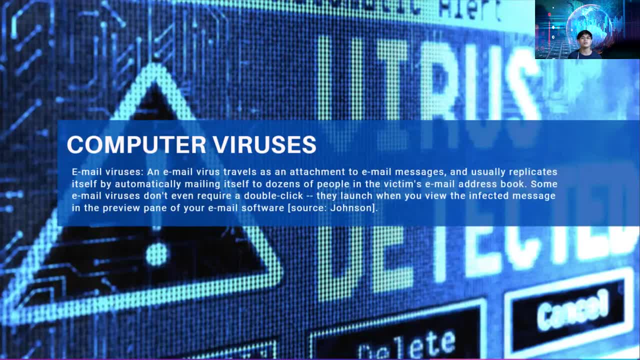 So it's very important that when you click, When you receive emails, and click each content, you must not just subscribe to any other sites And do not just subscribe to any other sites that are you know that are not legit or legit. 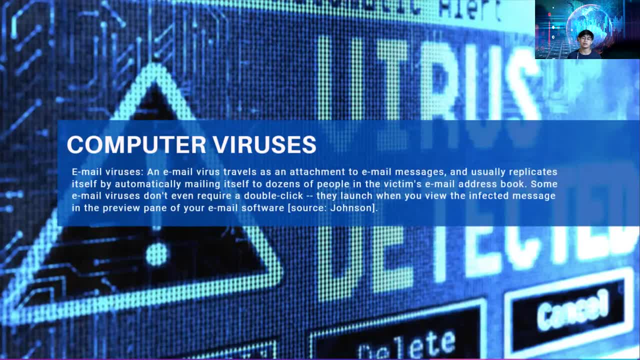 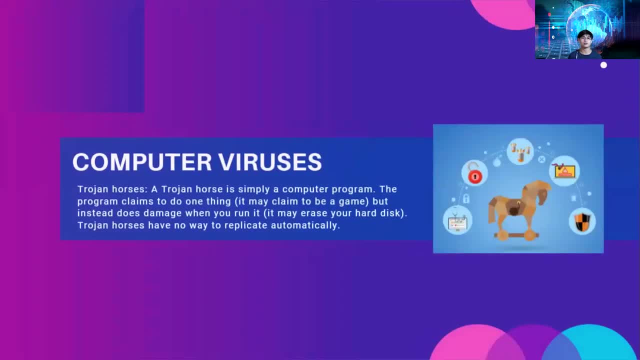 Okay, Because it's possible that you might get attacked by a virus. Next, Trojan Horse. So the Trojan Horse is simply a computer program. The program claims to do one thing. It may claim to be a game, But instead does damage when you run it. 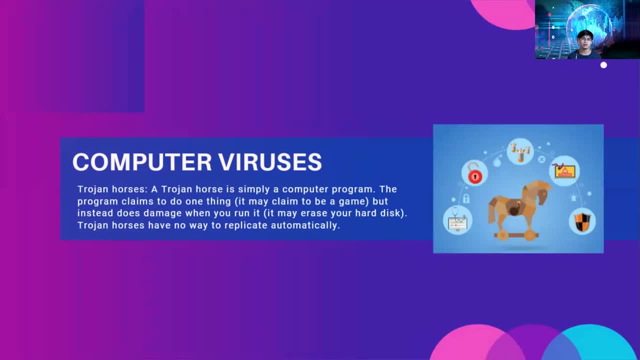 So it may erase your hard disk. Trojan Horses have no way to replicate automatically, So again it is something like a computer program. Okay, Now, if you let it run it will become a virus. Okay, So again it may corrupt or erase your hard disk. 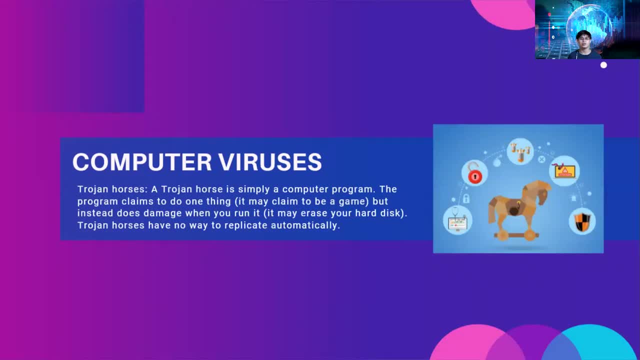 So if, for example, you got your hard disk, you lost your data, so you have to open an application and then it has Trojan Horses and then a cause of damage. So it's very important also to be aware of the virus. 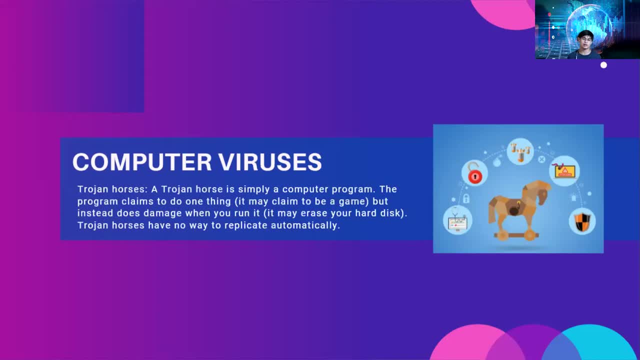 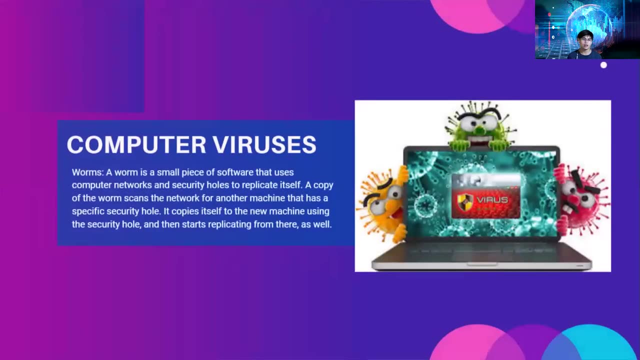 But don't worry, because this is what we will talk about in the next slides on how to you know how to solve these problems. Okay, The Worms. So a worm is a small piece of software that uses computer networks and security holes to replicate itself. 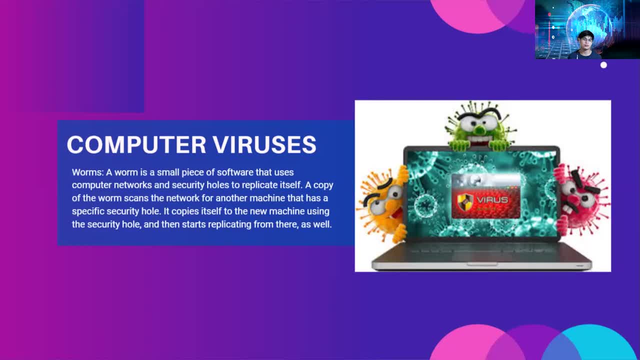 A copy of the worm scans the network for another machine that has a specifically security hole. So it copies itself to the new machine using the security hole and then starts replicating from there as well. So again it replicates itself. Okay, It is a piece of software again. 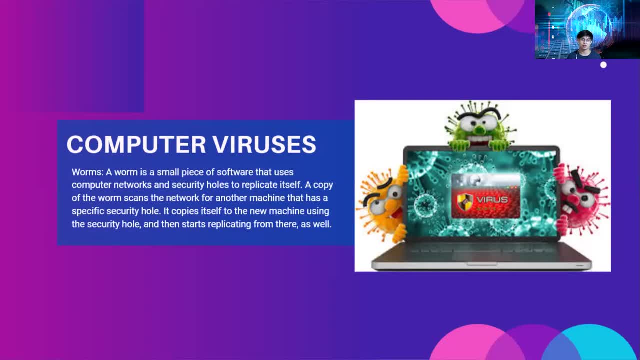 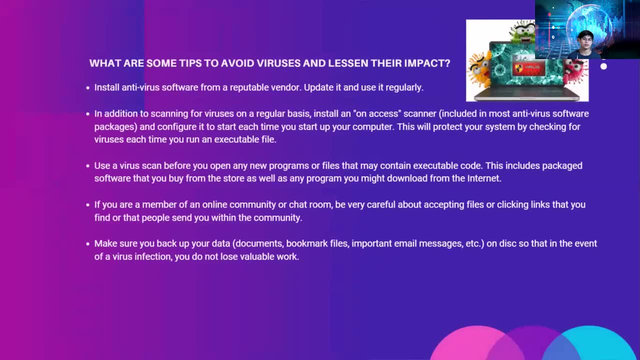 that uses computer networks and security holes to replicate itself. So be careful. Okay, So how to avoid the viruses and listen their impact? All you have just to do is very easy: lang: install antivirus software programs from a reputable vendor, Update it and use it regularly. 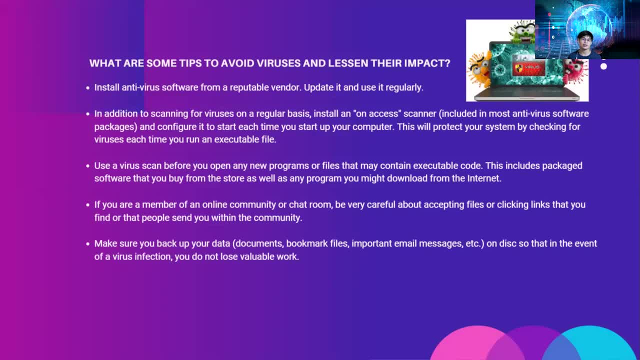 Diligid ka ba sa basta may install antivirus na diligid ka sa reputable vendor. Okay, It is possible. Nakata imong i-install sa imong computer is virus na mismo Diligid siya antivirus. So be very careful especially. 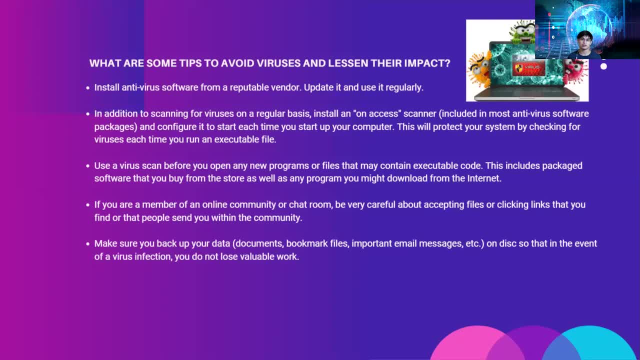 may uban. I believe na gagapang itag crack Mga crack. So there are a lot of free viruses So you have to find the crack. one Kata ng mga free And pwede na mong ma-install sa imong computer. 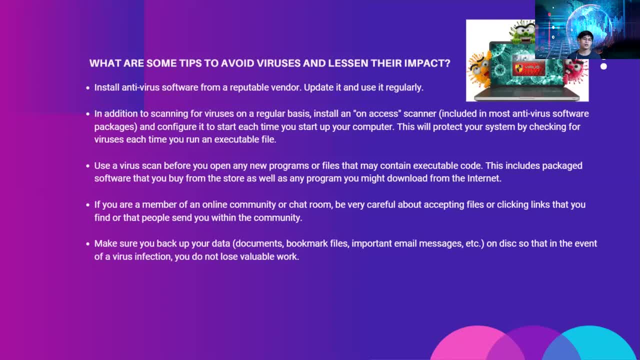 Okay, Nama kayo makita Okay. So, in addition to scanning for viruses on a regular basis. so after installing that antivirus program, you set its schedule for scanning for viruses. It could be on a regular basis or weekly, It's all up to you. 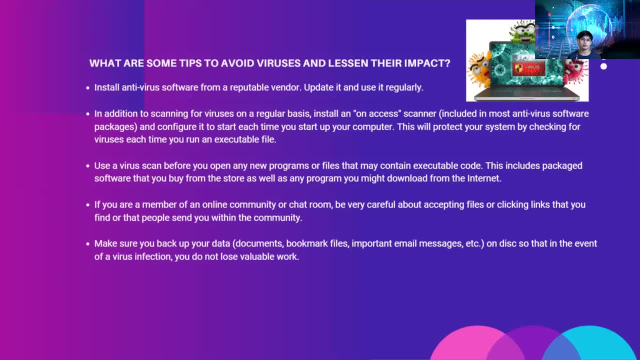 So install an on-access scanner included in the most antivirus software packages. So naana ni siya daan Pag open niyo sa antivirus. you just click the scan, So this will protect your system by checking for viruses each time you run an executable file.